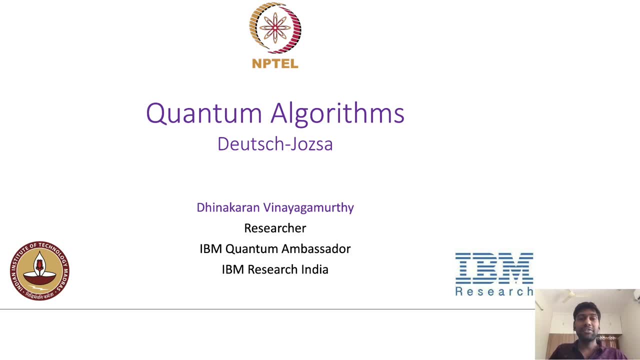 Okay, And there will be a two parts in week 3.. First is the coverage of Deutsch-Jozsa algorithm and the second part will be the coverage of Grover's algorithm. I will be doing the first part on Deutsch-Jozsa and I am Dhinakaran. I am a researcher in the IBM India research. 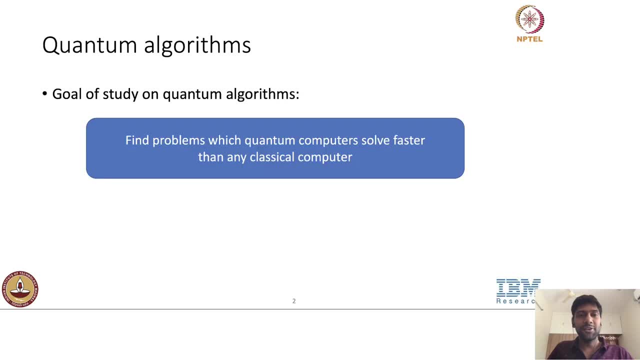 lab and I am also an IBM quantum ambassador. Okay, Let us take a step back. So why would you want to study about quantum algorithms? What can be the main reason? Because we already have classical computers which can solve many interesting things and sometimes like beyond our imagination, right? So why are quantum 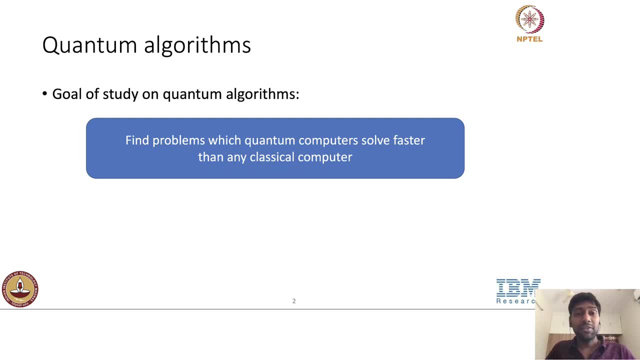 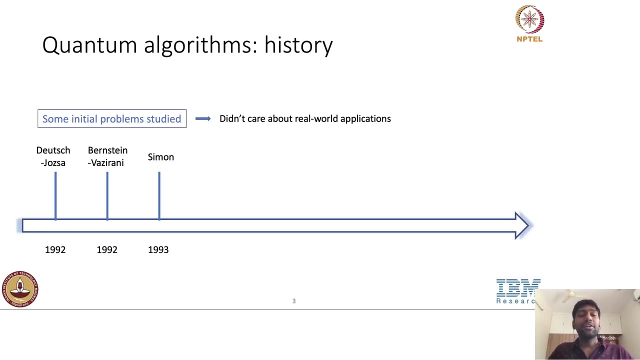 computers interesting. They are interesting only when they can do something which can be faster or it can provide a better quality solution than what any classical computer can provide, right, Okay, So when this research on quantum computing started in late 80s and early 90s- the initial 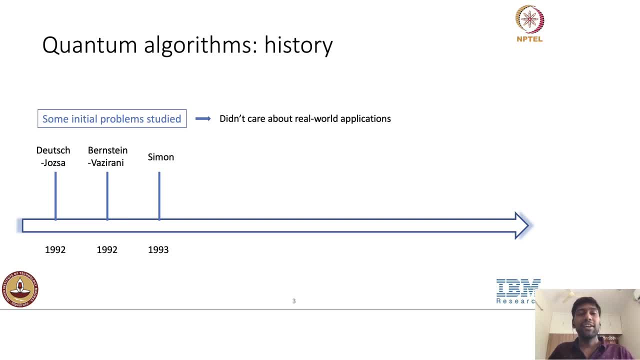 research was just. people are curious about finding one problem for which quantum computers can do provably faster than any classical computer. right Initially they did not really care about a real world application. To be honest, in 1990s, even for classical computers, 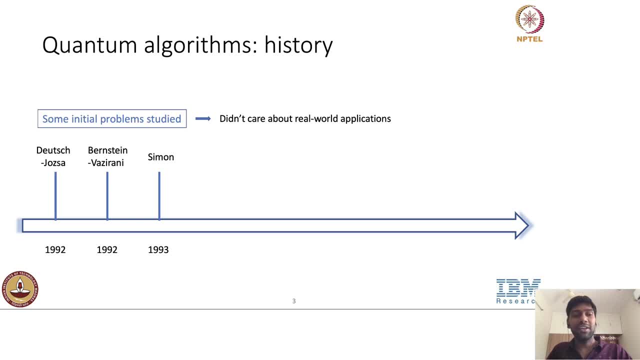 there were tons of any. there were not any interesting real world applications as we see today. right Back then people were just at least coming up, are interested in coming up with some problem and for which quantum computers can do faster than classical computers. 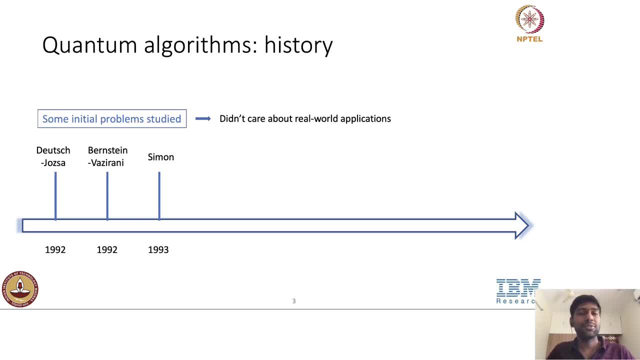 and indeed the initial problems that were studied were toy problems. And one more interesting point is that at that point there were not even a consensus whether quantum computers are faster than classical computers. Okay Right, In fact Dan Simon and this advisor did not believe that quantum computers. 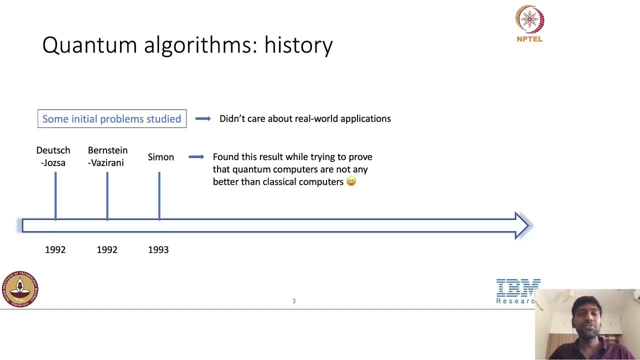 are faster. So Simon set out to prove that quantum computers are not any better than classical computers, and he found out an interesting problem for which quantum computers can be exponentially faster than classical computers in some sense, And indeed that formed a strong foundation. 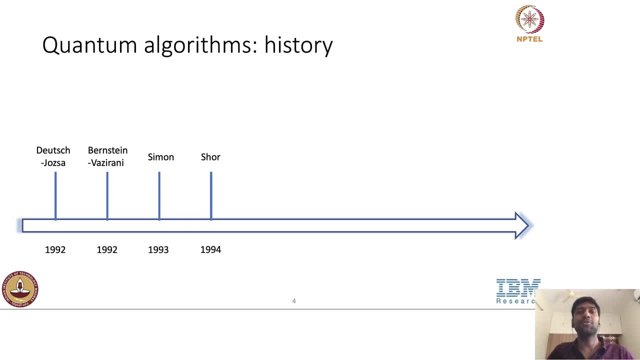 So for Schar's algorithm, which is a breakthrough for quantum computing because for the first time for a problem of real world interest, it is shown that quantum computers can do much faster than the best known classical algorithm. It is a Schar's algorithm for prime. 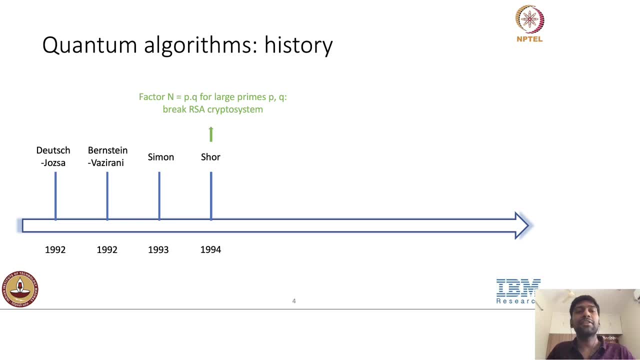 factorization, where Peter Schar showed that, given a product of two numbers which is the basis of four numbers, given a product of two numbers which is the basis of four numbers of modern cryptography, he showed that quantum computers can break that, which means that 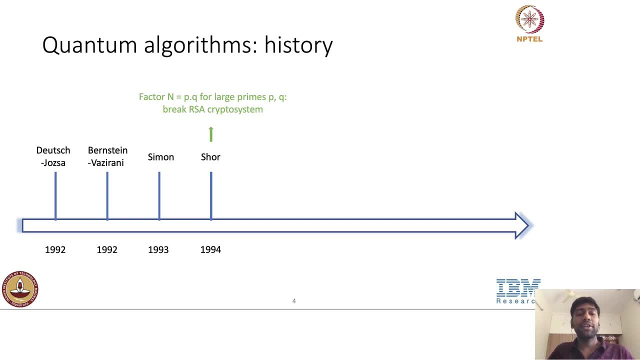 given a product of two primes, quantum computer can find the individual primes p and q, But this forms a basis of RSA cryptosystem, which assumes that it is hard for any classical computer to do this factorization, And hence we have built cryptosystems for quantum computing. 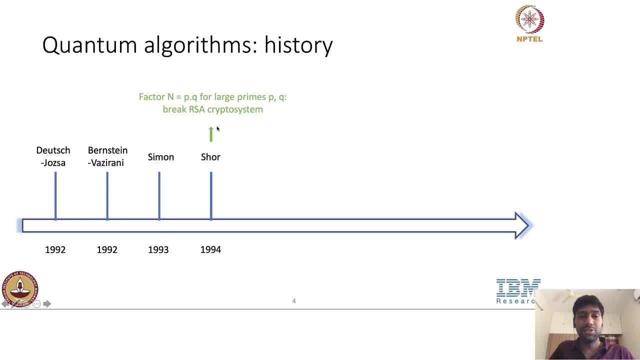 Okay. We have built cryptosystems on top of it and it is used widely. So Schar's algorithm gained a lot of attention, And after that we have had many interesting real world problems come up for which quantum computers can do faster. So for instance, this Grover's algorithm. 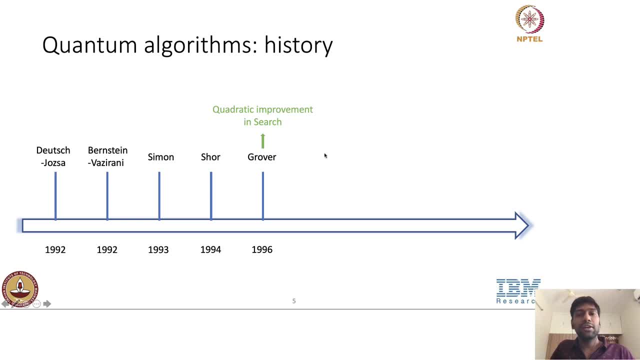 for generic search, which said that there is a quadratic improvement for quantum computers over classical computers. Okay, And from 90 years, in the current decade or the previous decade, we have started to see quantum algorithms for general optimization problems. And in 2016,- interesting thing happened. 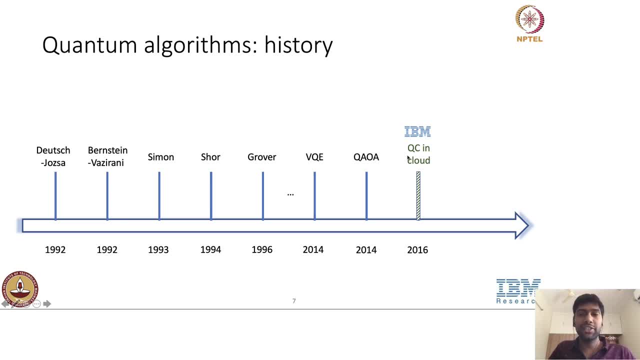 that quantum computers are not just restricted to labs and a handful of people. it is available to everyone to be used in cloud, which IBM first introduced in 2016 for quantum computers, And after that we have started seeing a plethora of concrete real world use cases. let us say: 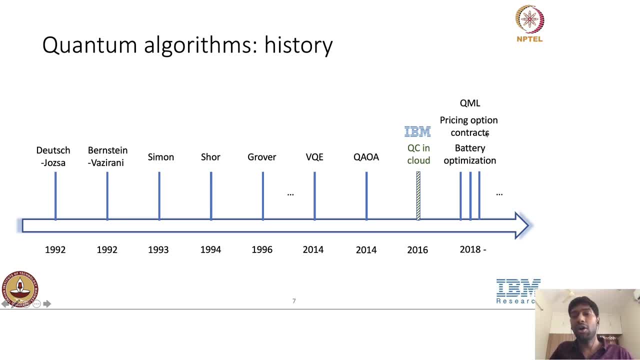 in battery optimization or the finance industry for pricing some contracts or in general in quantum machine learning. new research has started happening and results being shown for concrete real world problems in the last few years. To start with we will focus on the Deutsch-Joseph problem. 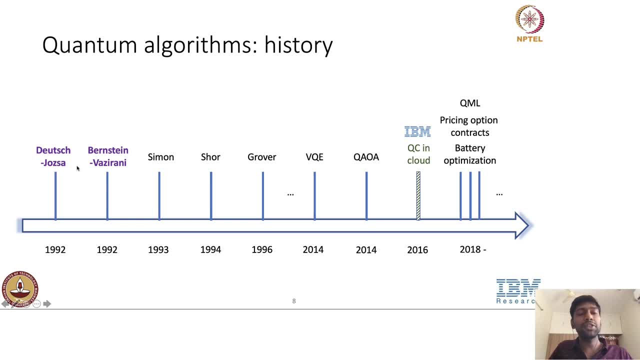 And give a brief glimpse of Quentin Vazirani problem. As I mentioned, these are tall problems, but this gives a good idea of the fundamental building blocks, a quantum algorithms use in the primitive stages, and then how these will get built. we will start seeing one by one. 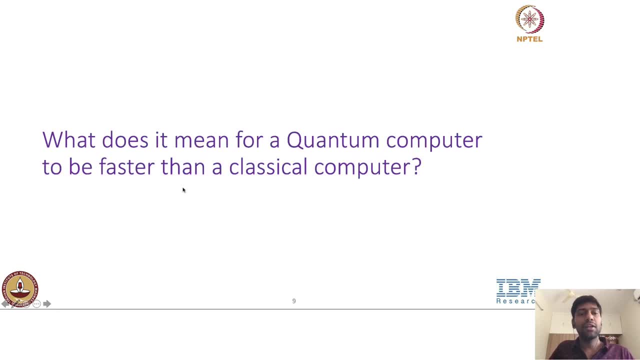 in the next few lectures. Okay, Before we go into the algorithm, let us first try to understand. what does it mean for a quantum computer to be faster than a classical computer? How do we say that this is fast and this is probably slower to solve this specific task? Let us now look at different 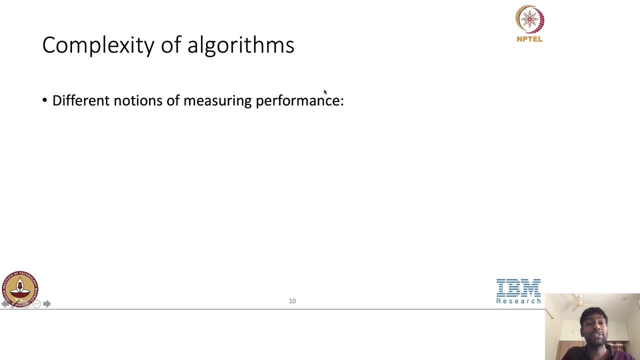 ways of measuring the performance, or it is called the complexity of algorithm. The most natural one is called the computational complexity, which measures the total computation time taken by the algorithm to solve the problem. The computational complexity to capture the maximum space or memory RAM plus storage that. 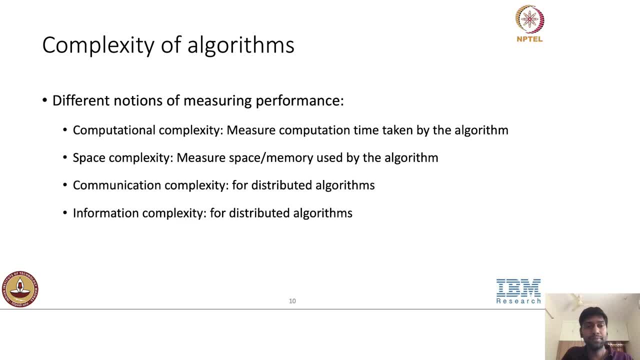 is required by the algorithm at any point of time. For distributed algorithms which involve computation between different clusters, communication complexity, information complexity can also be used. But to differentiate the complexity of two different notions of computing, query complexity, Okay. So query complexity seems more natural. So query complexity. what it says is that: 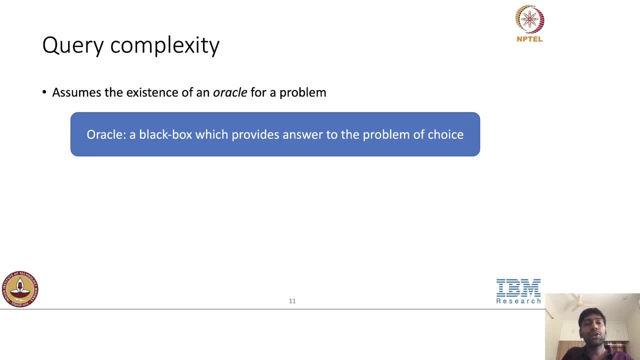 these algorithms. they also have access to a black box called an oracle, which has a function embedded in it, And whenever this algorithm that we are interested in it wants to solve that specific function, it can just provide an algorithm. It can just provide an query to this oracle and get back an answer. So this is a theoretical. 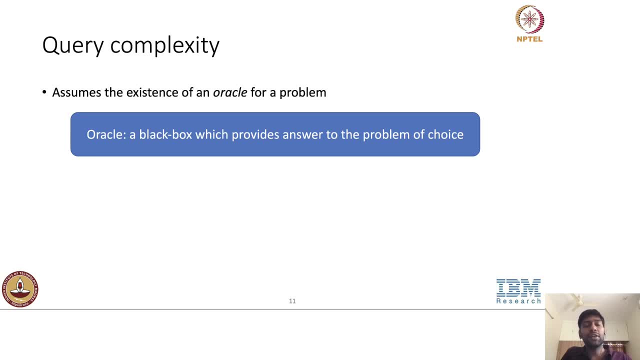 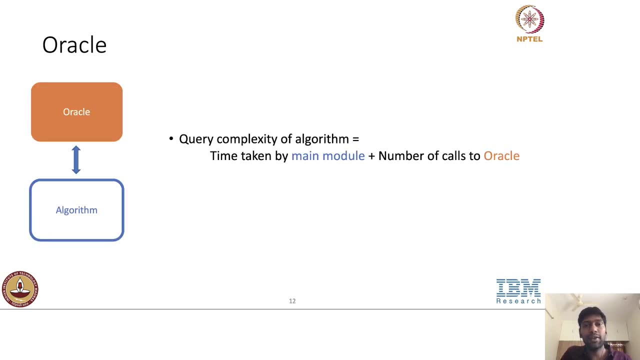 abstraction that is used to easily differentiate between two different kinds of algorithms. Okay, So to recap a query: complexity of an algorithm is time taken by the main module of an algorithm plus the number of times it calls the oracle. So this abstract notion, I mean, it is just 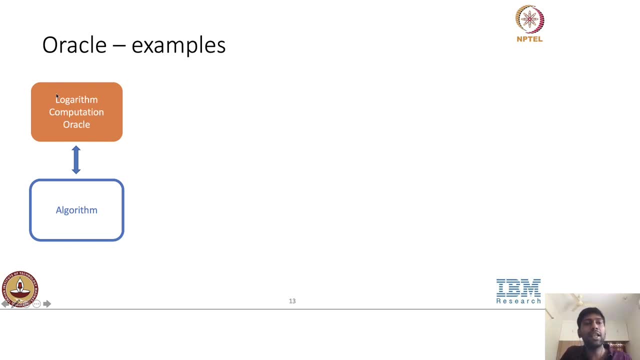 example, the oracle can be just as simple as computing the logarithm function, or it can be solving a linear program. It says that I mean, given a set of constraints, you find an input such that some substitute of constraints are minimized on that set of values, Or it: 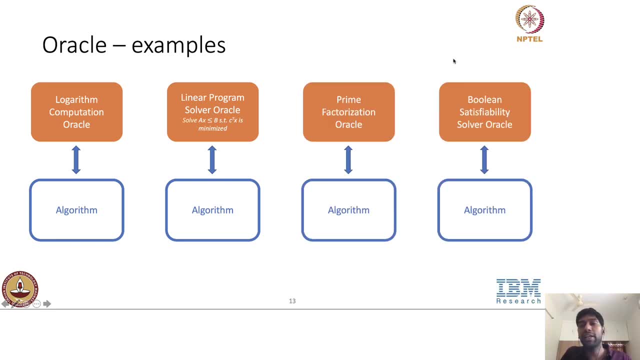 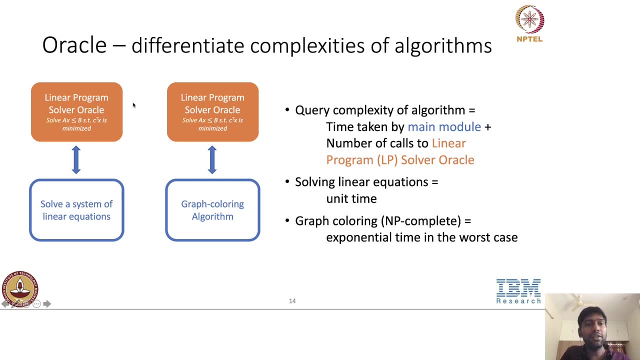 can be more powerful, like a prime factorization, or it can even be something like solving NP problem, But the main usage of this oracle is to of the subtraction of oracle is to differentiate the performance of two different functions or classes of functions which are hard to. 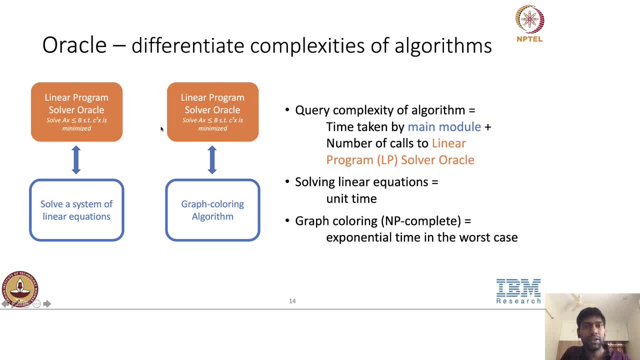 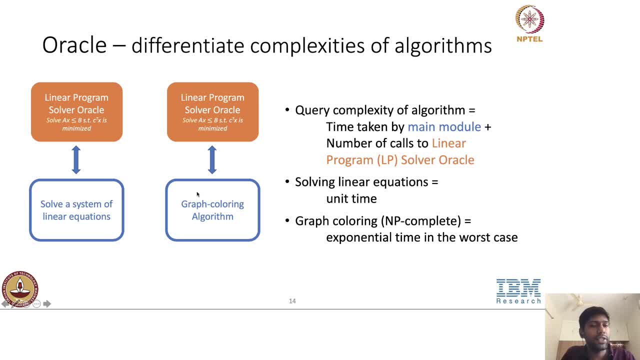 We want to solve a system of linear equations like: given a set of equations, you want to get a solutions for it. If you have access to this linear program, solver oracle, you just make one query to this and then solve. So the complexity of this is unit time In contrast. 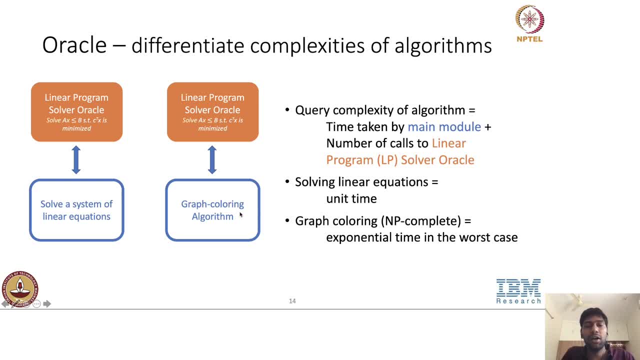 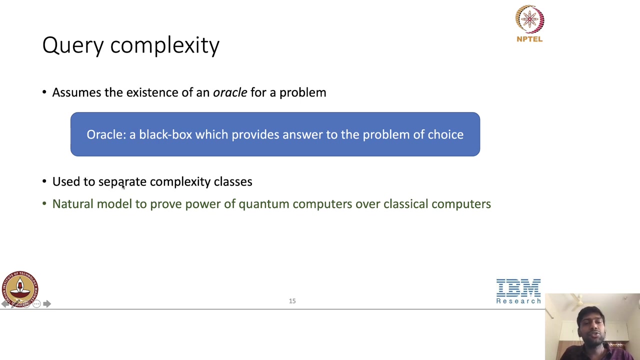 let us say we want to solve the graphical ring problem, which is an NP complete problem, is the best known algorithm for now. It takes exponential time to solve this, even if we have access to this powerful enough oracle of solving a linear program. So to summarize, query complexity is the complexity that is used to separate the performance of 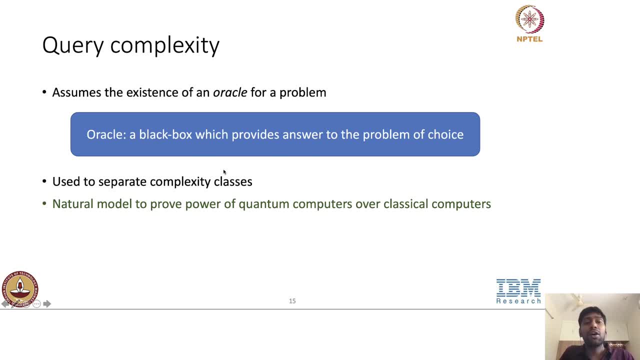 two different classes of functions or complexity of two classes of algorithms, And this is a natural model that researchers have used to show that quantum computers are more powerful than classical computer. So now, this is the background, this are all the background that we require before we go into a first quantum algorithm, which is the Deutsch-Josa. 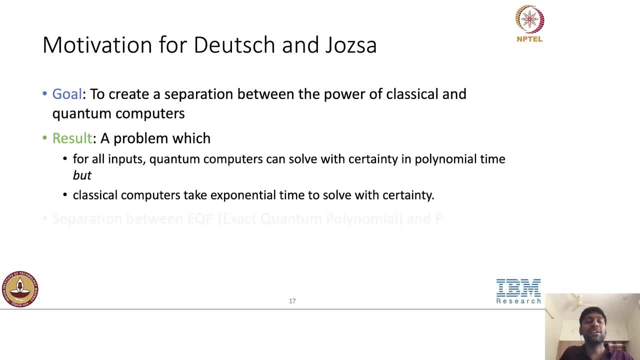 algorithm. What is the motivation for this algorithm? or at least we will see. what is the motivation that Deutsch and Josa had to come up with this algorithm. As a mentioned in the initial part of the presentation, their goal was to create a toy problem which. 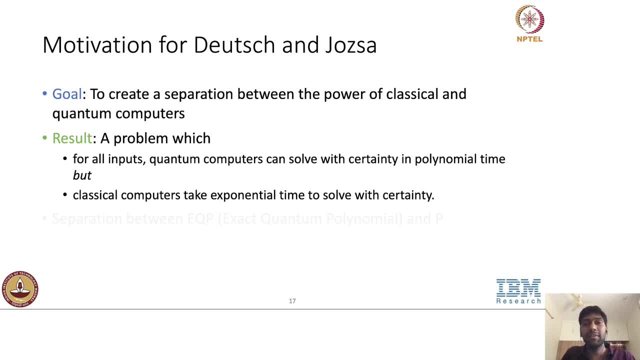 quantum computers can solve quickly, but classical computers, even the most powerful ones, should take a lot of time to solve. So their goal was to create a separation between the power of classical computers and quantum computers. and they came up with a particular problem which, for all inputs, quantum computers can solve with certainty in polynomial time. but 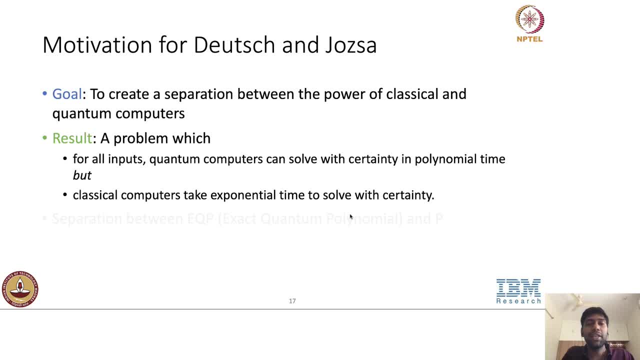 classical computers will take exponential time if they want to solve with 100 percent certainty. For those who know, it is a separation between the complexity class P and the complexity class exact quantum polynomial. but if you do not know about it, just skip it, it will. 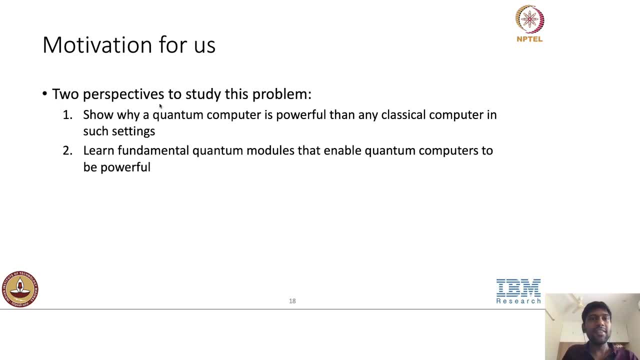 not be useful for the rest of the presentation. That is their motivation to solve. but what is our motivation for the rest of this part of the lecture? to study Deutsch's Algorithm. It is twofold. First, it is the same as theirs. 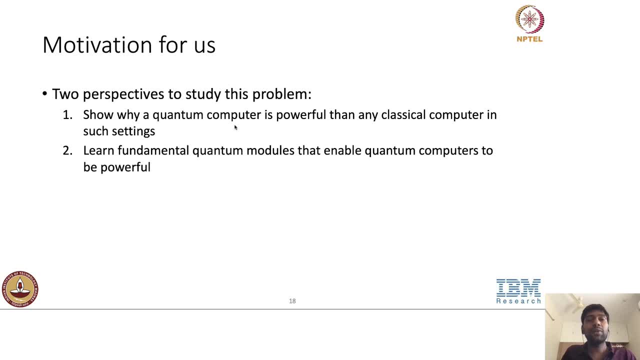 it is the first time we will see why a quantum computer is more powerful than any classical computer. but we also have the second motivation, to look at some of the fundamental quantum modules that will help us solve this problem. So let us start with the first motivation. 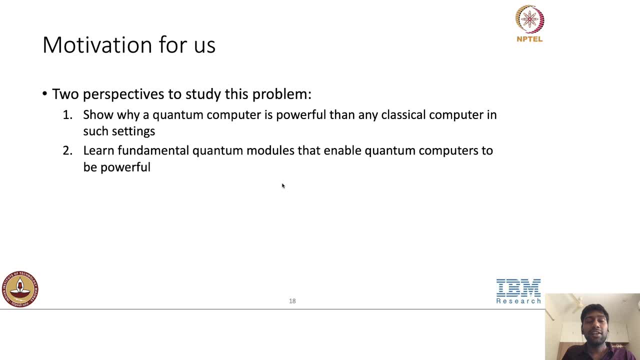 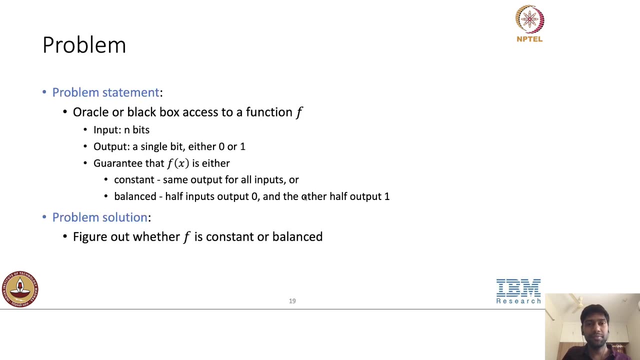 The first motivation will be used in this algorithm, which enable the quantum computers to be powerful. So we will use this lecture to also understand the fundamental quantum modules which will be used in quantum computers. So I told you that there is a particular problem that Deutsch and Djoser came up with, for which quantum computers can solve very 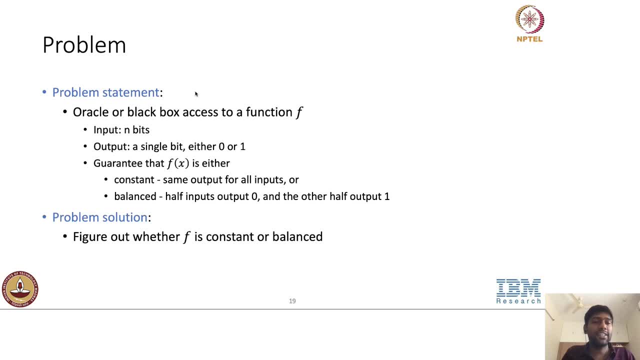 fast, But classical computers will take exponential time. So this is the problem. So the problem is that the functions, we are given an article, that is a black box axis to a particular function, f, with these guarantees. This function has a guarantee that it takes in n bits as input and the function will output. 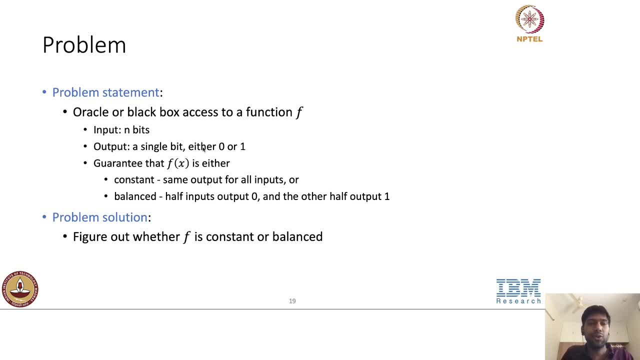 a single bit, 0 over 1, with a guarantee that f of x is either constant or balanced. So what that means is we know that this function either outputs the same value for all inputs or it is a balanced function, which means half of the inputs will output 0 and for the other half of the inputs 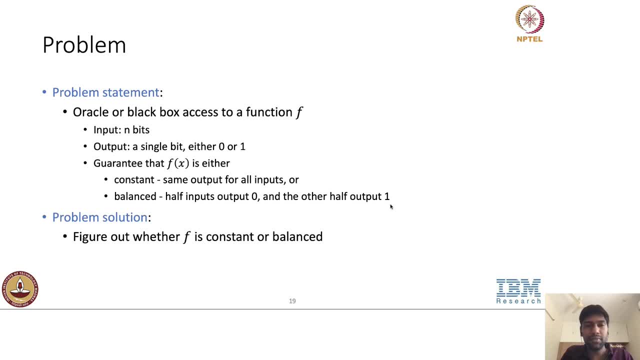 this function will output: 1.. Note that we are given black box access to this function, and the goal that Deutsch and Joza wanted a classical computer or a quantum computer to do is to figure out whether this f is constant or balanced. So we know that it is one of. 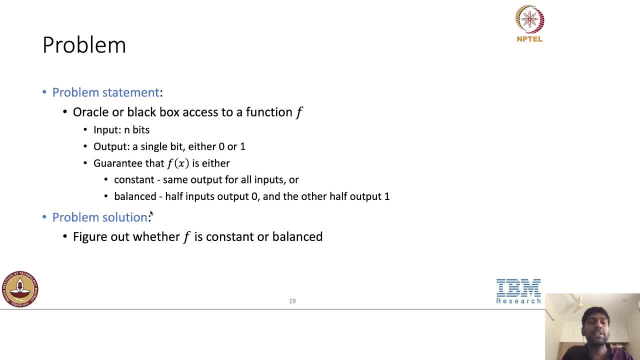 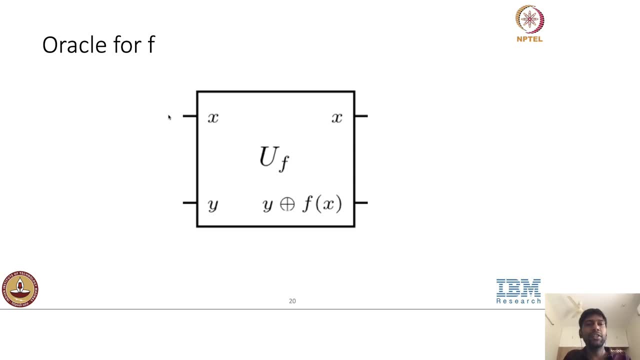 the two. We want to know with 100 percent certainty if it is constant or balanced. So now you that we are given an oracle or a black box access to this function f, So we do not know what the concrete function is, but we can give a set of inputs and get a set of. 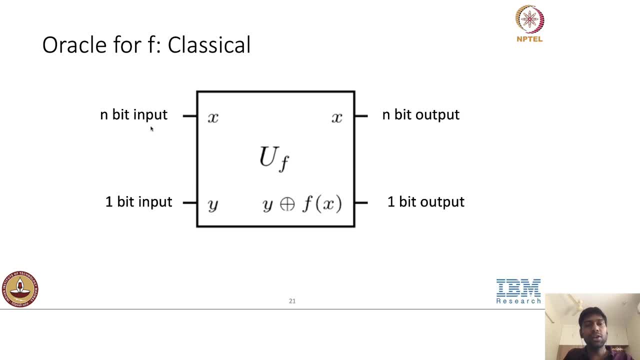 inputs. So this oracle- if it is a classical oracle it will get- it can take an n bit input plus another 1 bit input and then it will get the actual input, x as such, and the output of this function is embedded in this last 1 bit, that is, given y and x as input, the output will 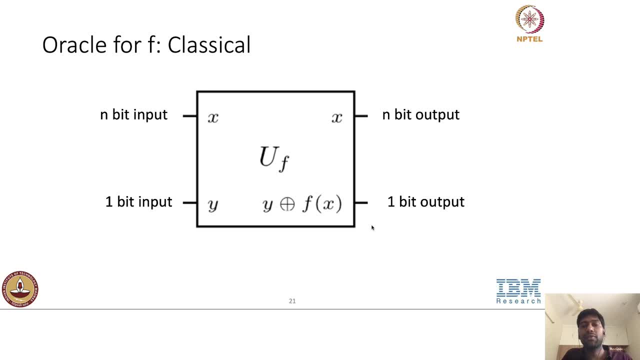 be x as such and y xor f of x. So, the last bit from the last bit, we can check the output of the function embedded in the plan The way we. this is the way we set it up because would have, if you remember from the first, 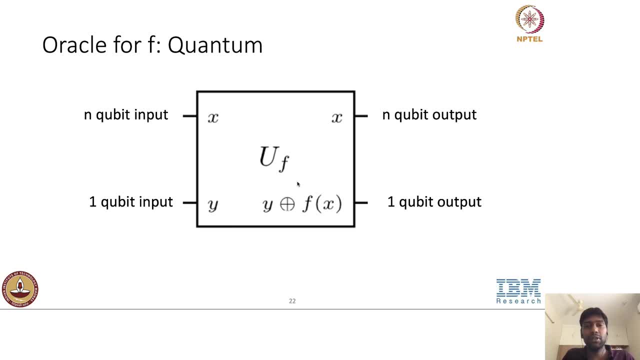 lecture. we know that the quantum computers have reversible computation, So we want the quantum oracle to be reversible. So this is an actual way of doing it. So if it is a quantum computer it takes n qubits. So it takes n qubits. 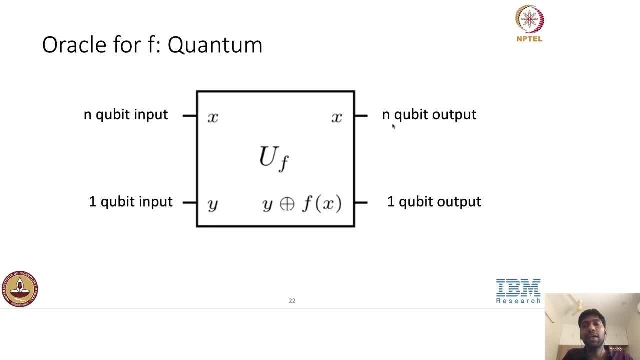 Plus 1 qubit as input and outputs, n qubits and 1 qubit, and the computation description is the same, except that it is a quantum module implemented. So now let us look at what is the classical algorithm to solve this problem. and right, remember that we need to find the 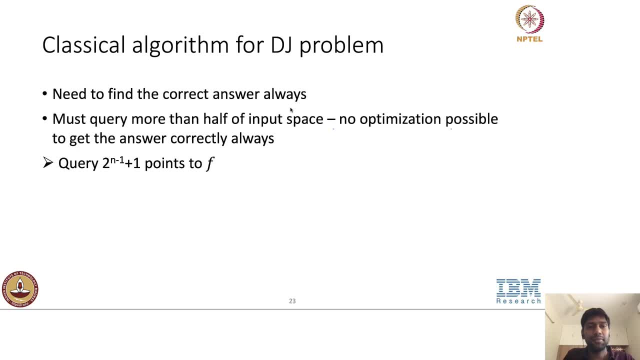 correct answer with 100 percent certainty. But if you think about it, given the black box access to this function, we need to query more than half of the input space to say with certainty whether this function is constant or balanced. So we want to figure out whether this function outputs the same value for all inputs or if 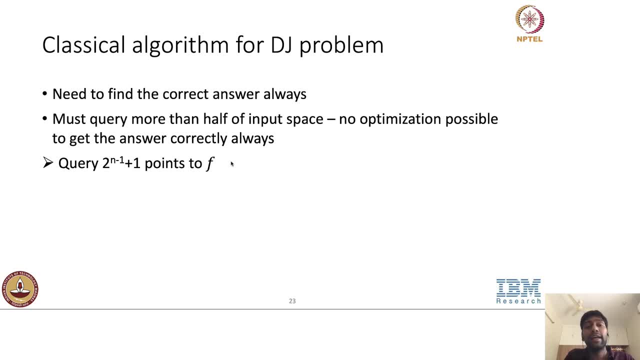 it outputs like half of the input space. So we need to find the correct answer with 100 percent certainty for half of the inputs output 0 and half of the inputs output 1.. But given that we want to solve with 100 percent certainty, we have to query at least half of. 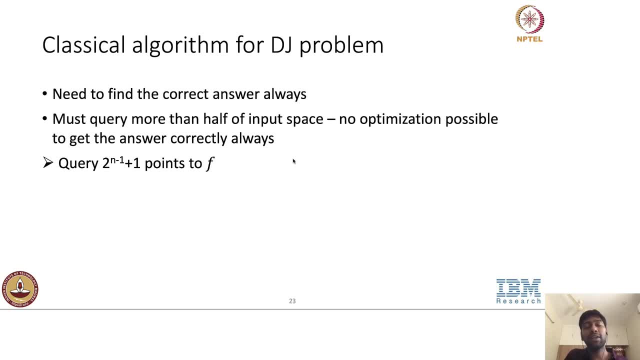 the inputs plus 1, because we might end up being unlucky and let us say, for the first half of the inputs, that is, 2 to the n minus 1 of the inputs that we query, We get the same output. that does not say anything whether this function is constant or balanced, because 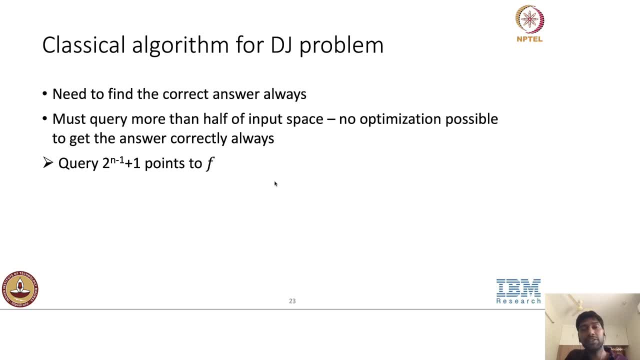 it could be that it is a balanced function which is so unlucky to not get the correct, I mean the different output for the first 2 to the n minus 1 inputs that we query, So to say the answer with 100 percent certainty to predict whether it is a constant function. 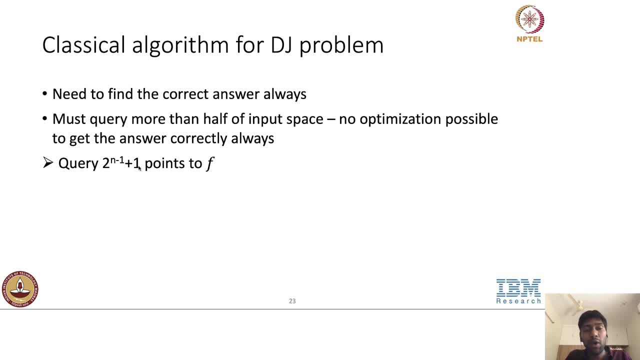 or a balanced function, need to query at least one point more than 2 to the n minus 1 inputs. So hence the query complexity for the classical algorithm is exponential in the input length n. The interesting thing is the quantum algorithm for the dial shows up problem solves this. 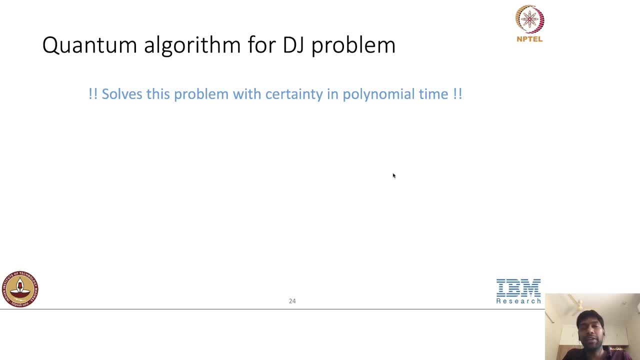 or predicts whether the function is constant or balanced in polynomial time. In fact, just with constant queries to this oracle, we can predict. We will now see how this works. We will get into the quantum algorithm part of it. So step 0 of the quantum algorithm, this is the input that we provide to the quantum 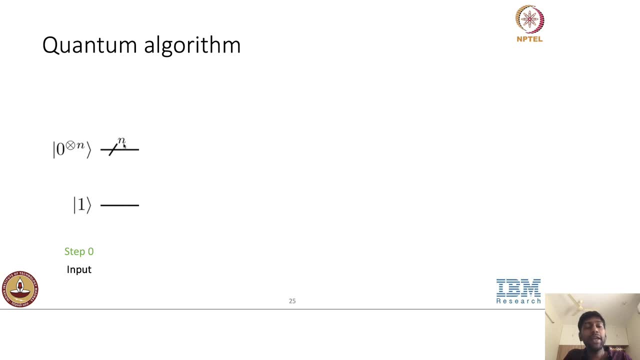 algorithm, The n bit, n qubit, part of the input. it is all 0s and the last qubit will take in a qubit 1 as input. Now step 1, the step 1 of the quantum algorithm for solving a dial. 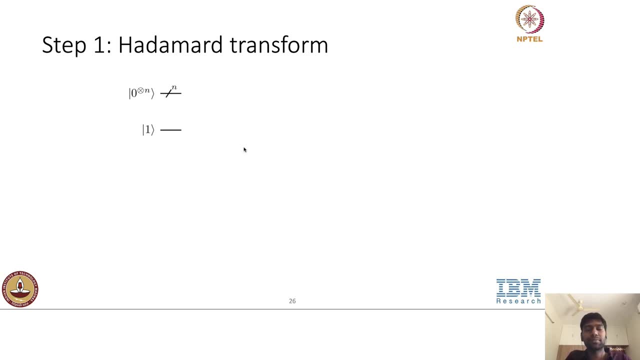 shows up. problem is applying the Hadamard transform. If you remember from the first couple of weeks, Hadamard gate is as follows: it is 1 over root, 2, 1, 1, 1 minus 1.. In particular, it transfers the 0 state into the plus state, which is 1. 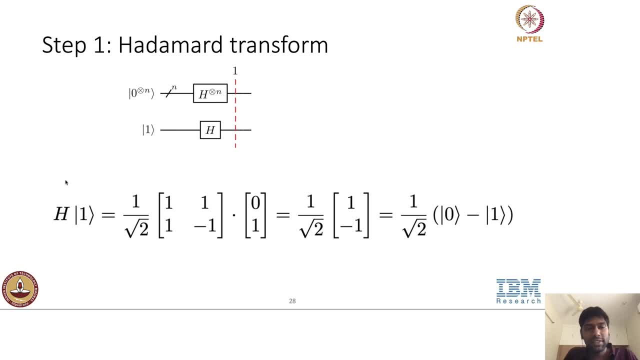 over root 2, 0 plus 1 and 1 state into a minus state, which is 1 over root, 2, 0 minus 1.. So we know that Hadamard transfers. Hadamard is a single qubit gate acting on a qubit 0,. 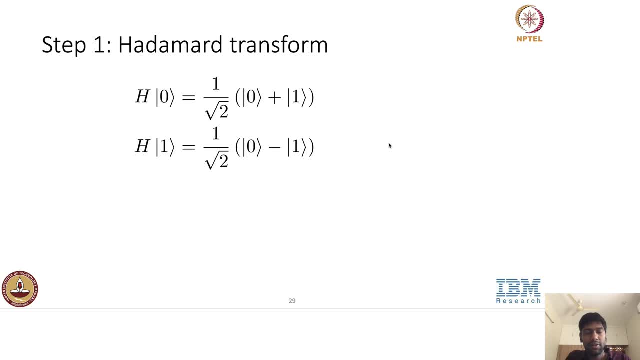 it transfers 0 to plus and 1 to minus. So to abstract it out, if Hadamard acts on a general gate, general qubit A, general single qubit A, we can see that the first qubit. it is always like it does not have any phases. 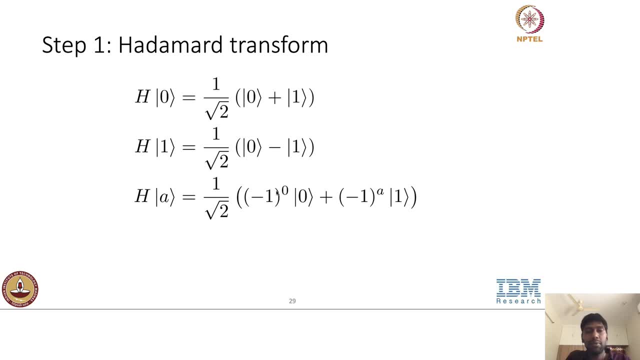 associated with it. So for corresponding qubit 0, there is a single qubit A. there is minus 1 to the 0, and if the input is 0, it is again 0, but if its input is 1, it is. 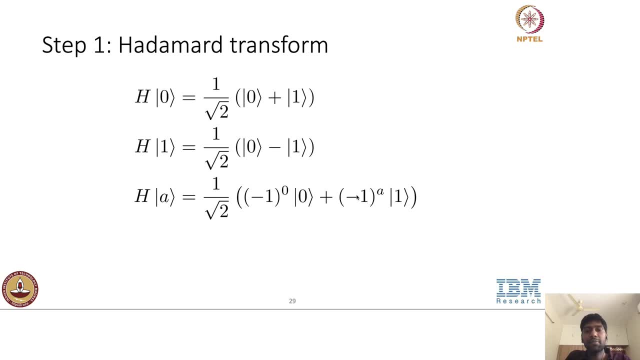 minus 1.. So we can generalize it and write it as minus 1 to the power. In fact we can bring these two together and then say that Hadamard, when it is applied on a general single qubit, A, is minus 1 to the power. A dot x, x. 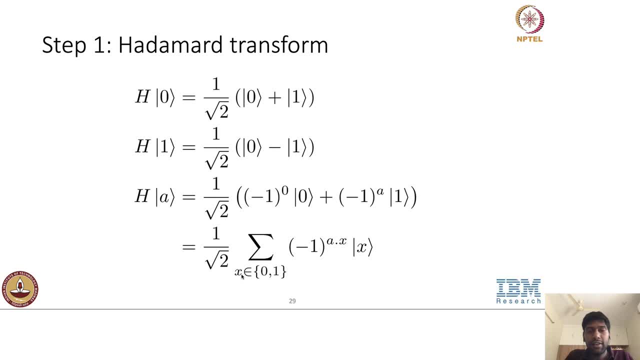 So just to see it again, when x is 0, it is minus 1 to the 0, 0, which is this. and if x is 1, it is minus 1 to the A dot. 1, which is A, and 1, which is this. 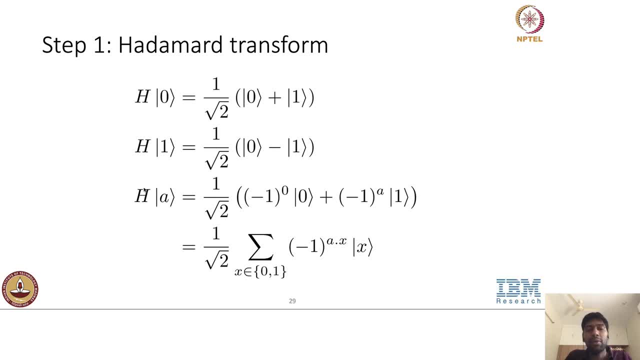 So for a single qubit. when Hadamard apply on a single qubit, we can easily see that it is written this way. I am not going to explain, but this generalizes, even when we are applying this H hat aqueles to the number one. What is happiness In which case? it is? 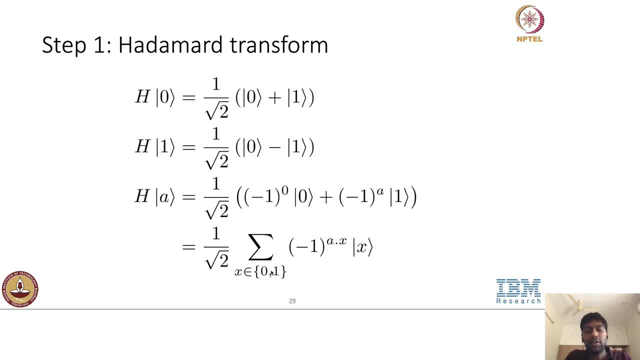 multiple Hadamard are applied on multiple qubits. So for a multi qubit gate, A multi qubit input, A, let us say n qubits for instance, When Hadamard is applied on those we get the same expression minus 1 to the A dot x, where A dot x is a dot product between A and 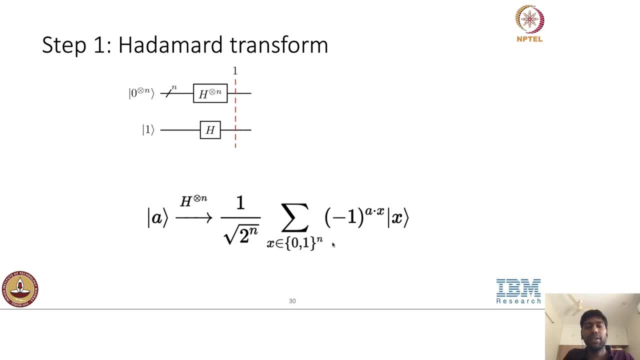 x and for all possible inputs x. In fact, this is what we will have as a first step of quantum algorithm. This expression we will use it later, but for the first step. it is easy to see because for the first register, so we have n qubits, all of them are zeros, So the input is let. 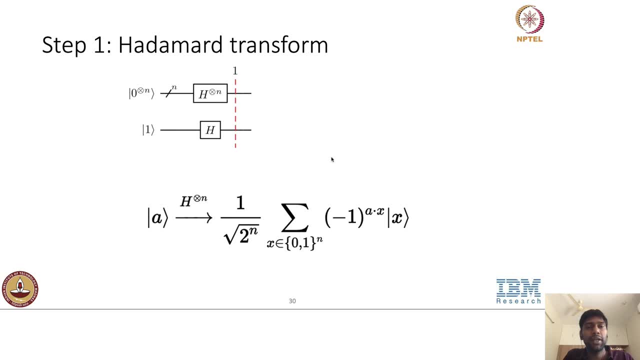 us ignore, like let us just focus on the first n qubits. qubits being applied for the first step, because we know that 1, when has a Hadamard, it becomes a minus. And also the for the first 10 qubits, when it is all 0s. it is just equal superposition. 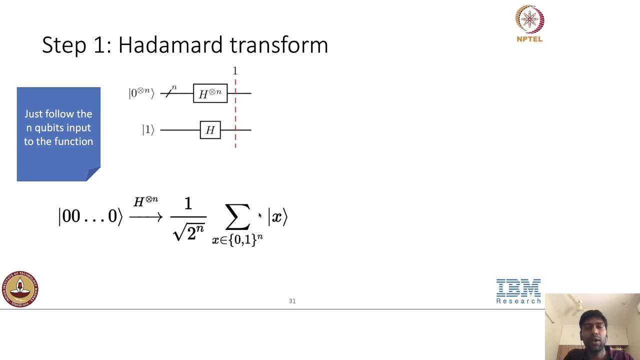 of all possible states, because minus 1 to the erodex is always 1.. So this is simple. this is the step 1, we have all 0 input in the first register and we apply Hadamard. we get equal superposition of all possible states. The second step is: 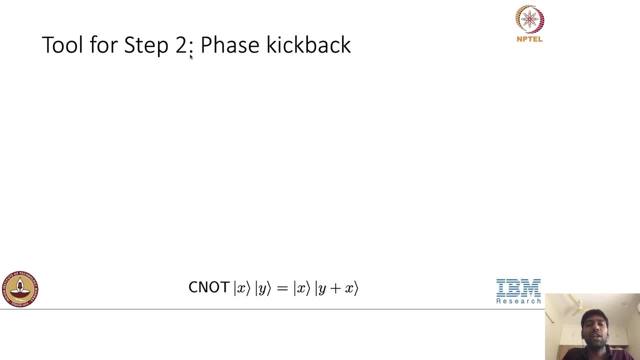 an interesting tool called the phase kickback that you will see in many quantum algorithms, The starting point. let me explain what phase kickback is. So the starting point for it is the CNOT gate. So CNOT, we know it is a 2 qubit gate, So it takes in, let us say, input. 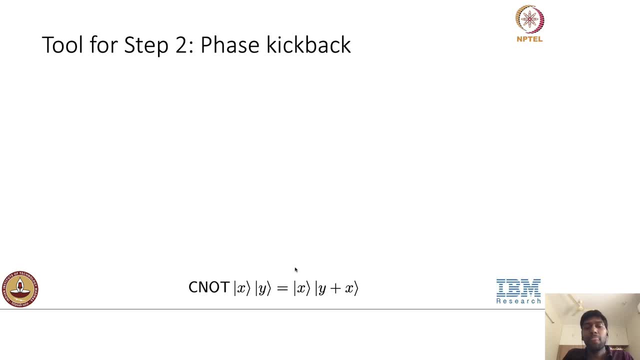 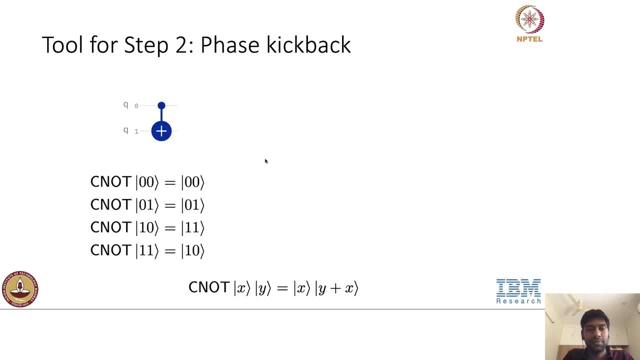 a 2 qubit gate where the output is x and y plus y- y. So to instantiate it, let us say that 2 qubits, q 0 and q 1, q 0 is a control and q 1 is a target. So this together: 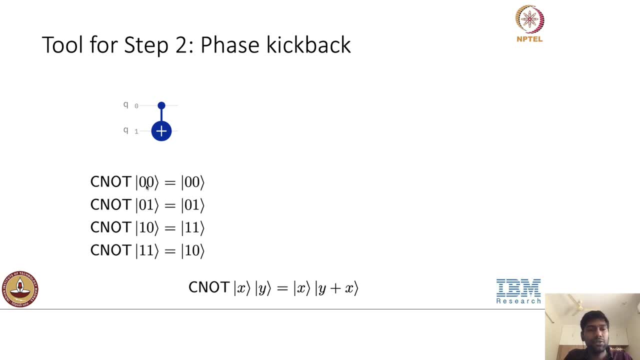 is the CNOT gate, CNOT when it is applied on 0, 0.. So I am saying 0 is q 0 and the first position is q 0 and second position is q 1.. So CNOT applied on 0, 0, 0, 0, 0,. 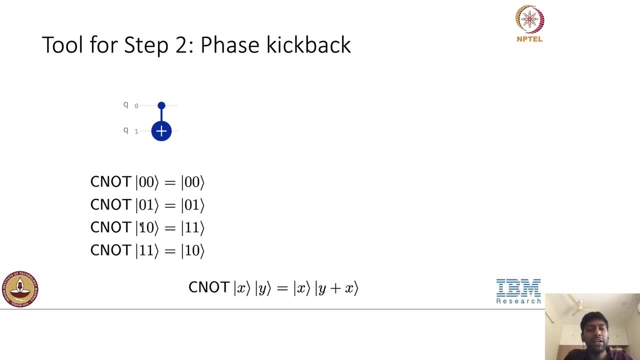 the control is 0, so target remains unchanged, But when the control is 1, the target is flipped. that is the property of a CNOT gate. But let us look at this thing. let us look at the Hadamard applied before and after the CNOT gate. When you work this out, the interesting 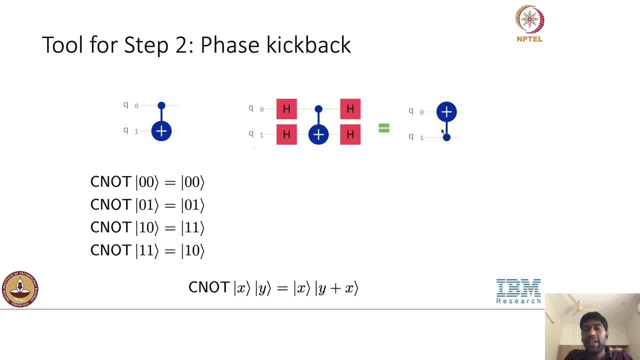 thing that you will see is the CNOT gate. it acts as if it is flipped. the control and targets are flipped if we have Hadamard applied before and after. That is here. when we have CNOT applied on the standard basis, the control target are like this, but if we have Hadamard, 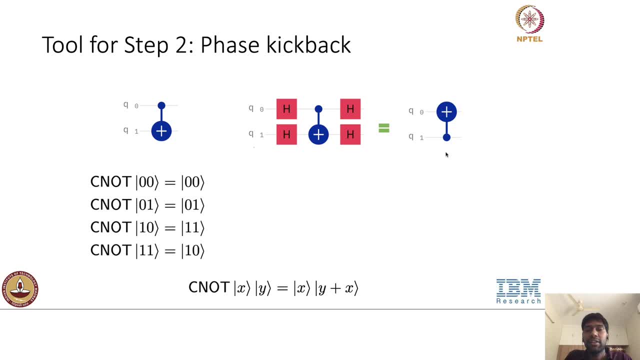 on. sorry, if we have CNOT on the Hadamard basis, then the effect of CNOT is flipped. You can work it out. but if you work it out, you will see that if we have Hadamard, so CNOT, Hadamard, 0, 0 will become 0, 0, but 0, 1 becomes 1, 1.. So it is as if the second 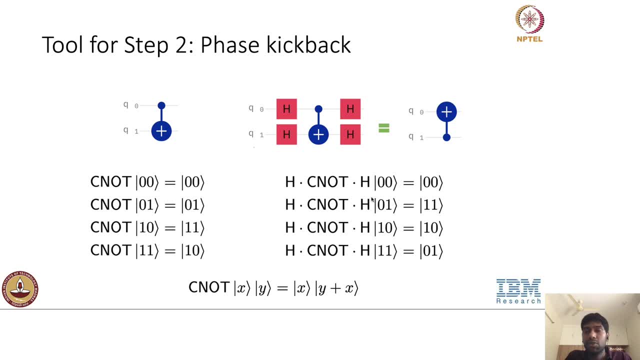 qubit is the control. So since the second qubit is 1,, the target gets flipped. so it is like this: So 1: 0 is 1, 0, because the control is 0, and 1: 1 becomes 0, 1.. So this is starting. 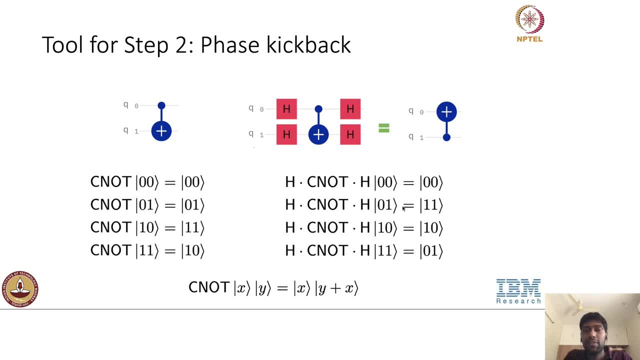 point to see the notion of phase kickback. Let me say a more explicit way of using phase kickback. Let us just look at the Hadamard. So essentially the standard basis converted into Hadamard basis by the time we apply. 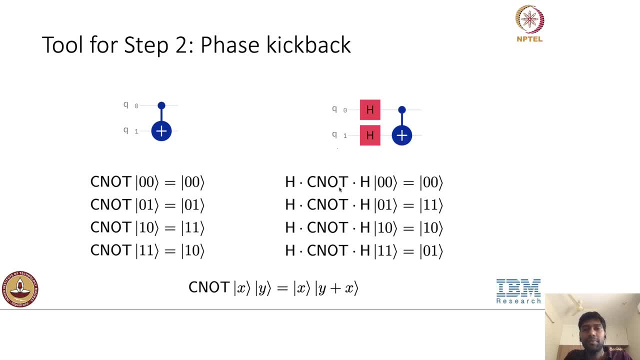 after we apply Hadamard, before the CNOT gate is applied. Now let us look at all possible inputs for q 0 and q 1.. Let us see what the impact is. So CNOT: we know that. 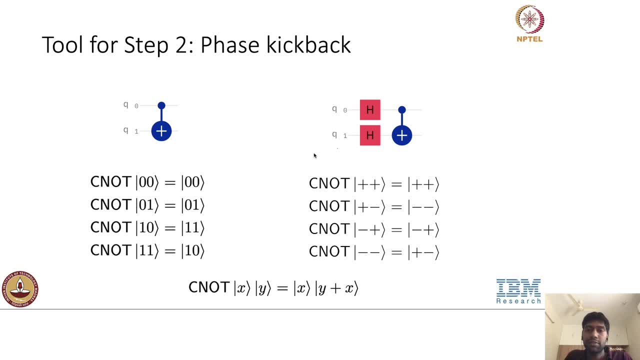 Like Hadamard on 0 is plus and Hadamard on 1 is minus state. So CNOT on plus plus gives plus plus, but CNOT on plus minus gives minus minus, and CNOT on minus plus gives a minus plus, and CNOT on minus minus gives a plus minus. So it is like if we have the second 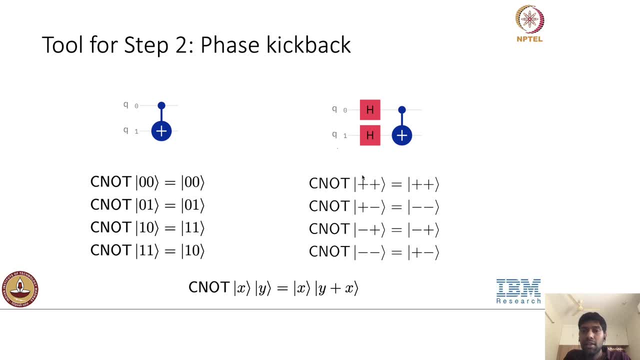 qubit as plus, the first qubit remains unchanged, but if we have the second qubit as minus, the first qubit gets flipped in the Hadamard basis. So it is a plus becomes a minus and minus becomes a plus. 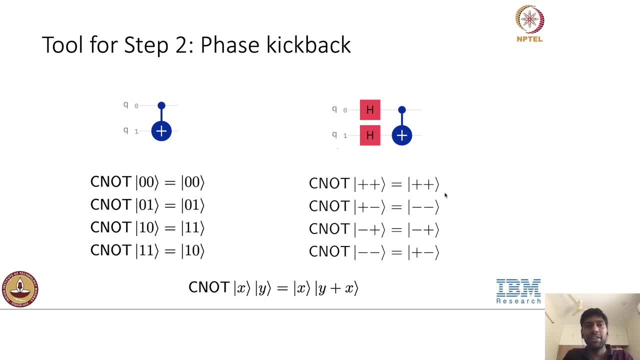 So, similar to how we derived an expression for Hadamard in the for the first step, we will derive expression similarly for this phase kickback. This is what we call a phase kickback. So if we have the phase a phase in the second qubit, that gets kicked back. 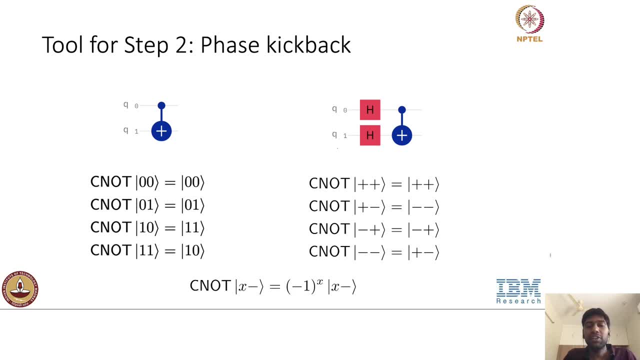 to the first qubit. So in general we will derive this expression. So CNOT on x followed by a minus will have this phase. that gets kicked back to the first qubit, minus 1 to the x. Let us derive this. 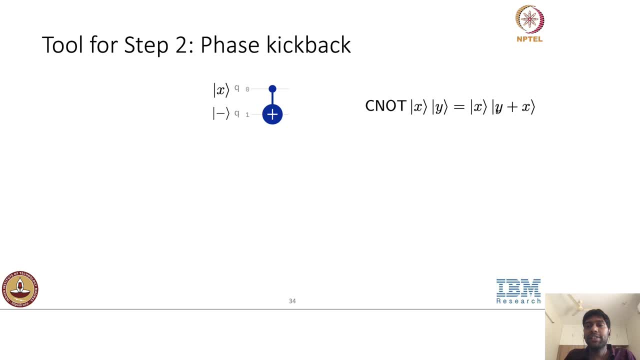 right. So we know that CNOT on x y is x y plus x. So what is CNOT on x minus? So what is minus Minus is 1 over root 2 ket 0 minus ket 1.. 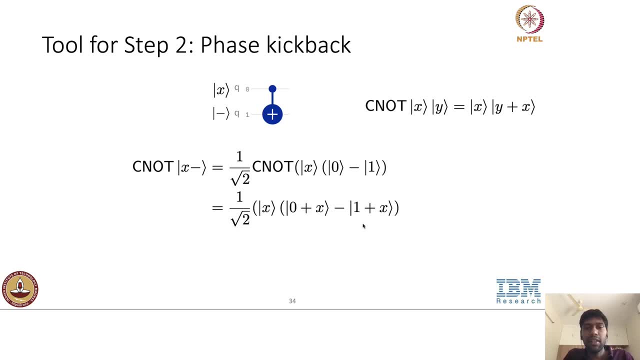 The first is unchanged. Let us just expand this. So right. So let us say: CNOT applied on 0 minus 1 is. from this expression we know that CNOT applied on 0 is 0 plus x, because the control is x minus 1 plus x. It is just this regular CNOT gate applied. 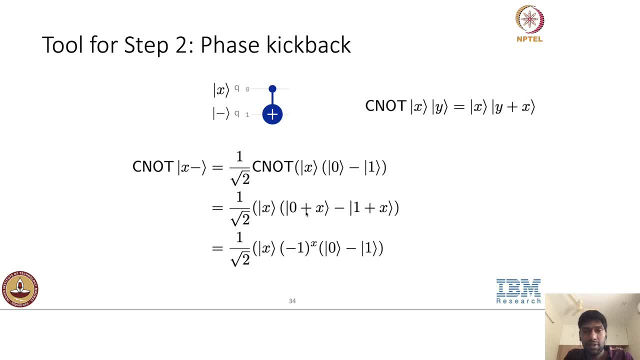 If you just look at this, this 0 plus x minus 1 plus x can be simplified as minus 1 to the x 0 minus 1.. So this is because if x is 0, then it is essentially 0 minus 1.. So this: 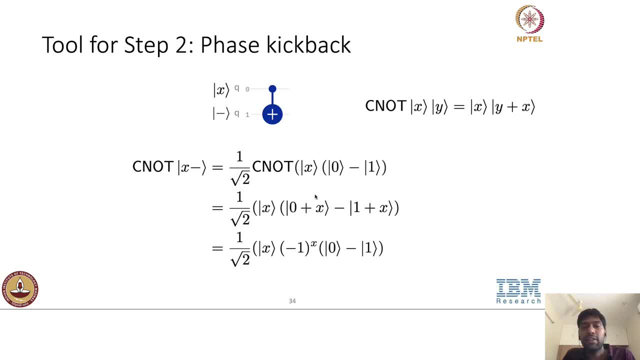 is unchanged. But if it is x is 1, then this is 1 minus 1 plus 1 is 0. So this is unchanged. So it is 1 minus 0, which can be written as minus 1 times 0 minus 1.. So essentially, 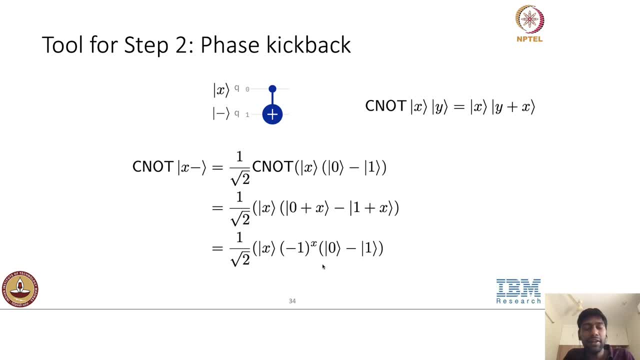 if x is, if the control is 0, then there is no phase that comes up. But if it is 1, then we have this term, phase minus 1, that comes up. But this minus 1 to the x is a global. 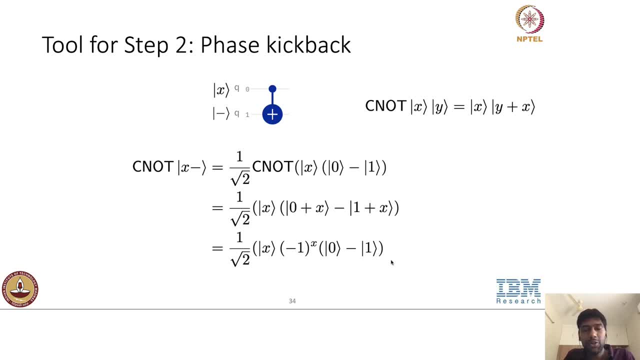 phase. So then we applied to either the second qubit or the first qubit. That is essentially the notion of phase kickback, Even though we started with the CNOT gate and x is the control. but if we have the second qubit as a minus, there will be a global phase minus 1 to the 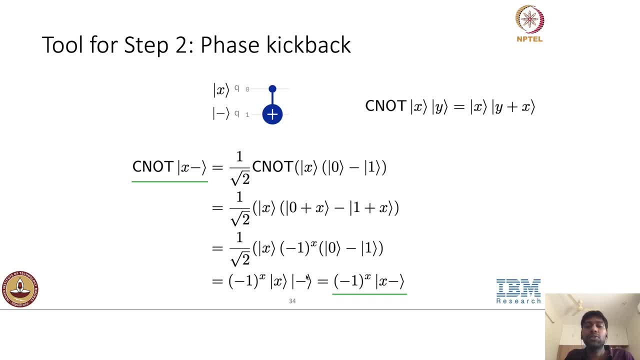 x that comes up And that can also be kicked back to the phase kickback. So this is the first qubit and applied on the first qubit, x. So CNOT of applied on x and minus will give minus 1 to the x x minus. So this is the expression that we develop Intuition. 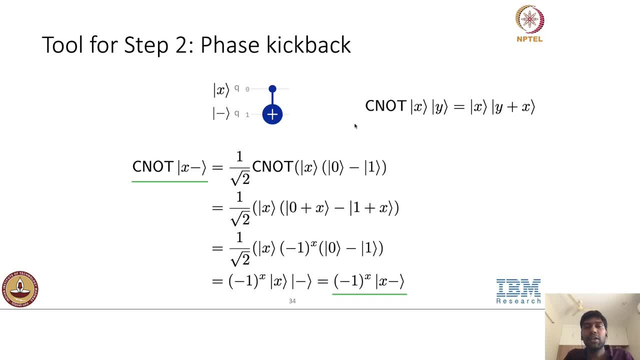 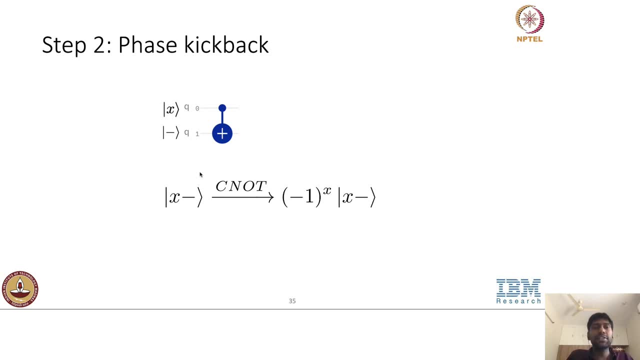 you can see from the previous slides, we have the Hadamard applied before and that, but this is the expression that comes up And this is when CNOT is applied on the first qubit. CNOT is applied when the first qubit is just x, but this can be more generalized. 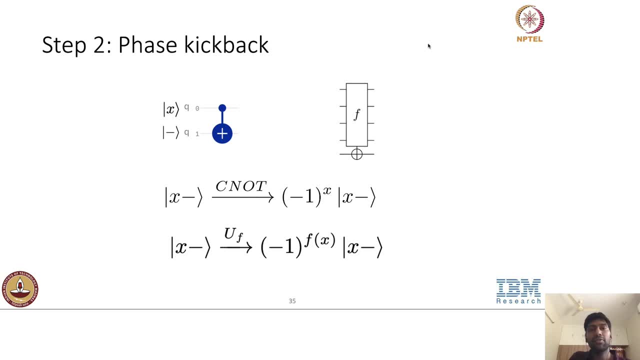 Even when, instead of a single qubit x we have a multi-qubit control. Let us say we have a function that is applied Like: this is the oracle that we had. We had an x and x here and we have y and it is y xor f of x. That is the oracle that we have. So if we 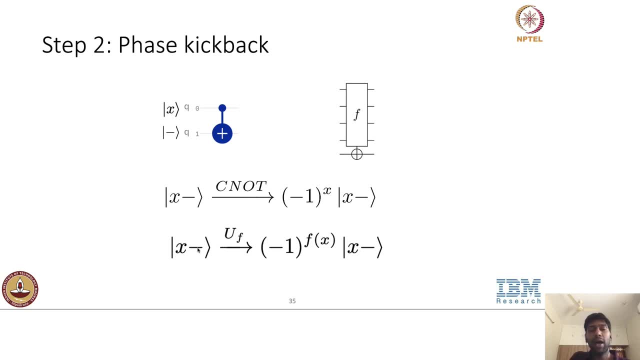 have this multi-qubit x and minus gate is passed through our oracle, the phase kickback property ensures that we will get this output minus 1 to the f of x as a global phase and x and minus. So this is the second step, phase kickback. So this is the oracle that we applied. 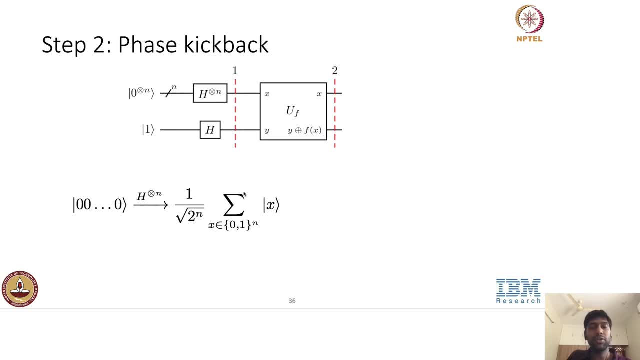 and the output of first step we got as 1 over root 1.. So equal superposition of all possible inputs. And now, when we apply the oracle u f, we will get this x. we will have this global phase. the phase kickback applied to x will have minus 1 to the power f of x. So 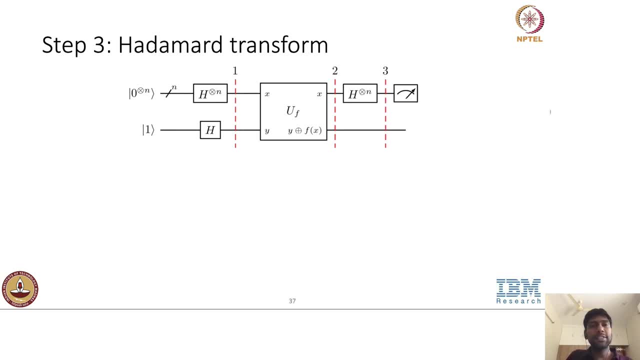 this is the second step. Now let us move to the third step, which is again applying the Hadamard transform. So this is where we will use the general expression that we have derived for Hadamard transform, which said that if you have Hadamard like, n applied. 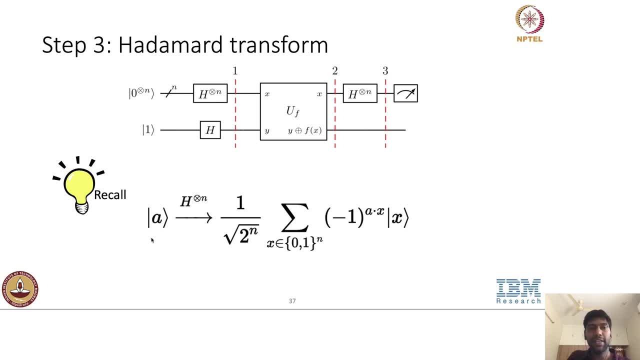 on n qubits. a. a is n qubit register. Let us say: if you apply Hadamard on n qubits, we will get this expression summation over all possible: x minus 1 to the power, a dot, x, dot. product between a and x and x. 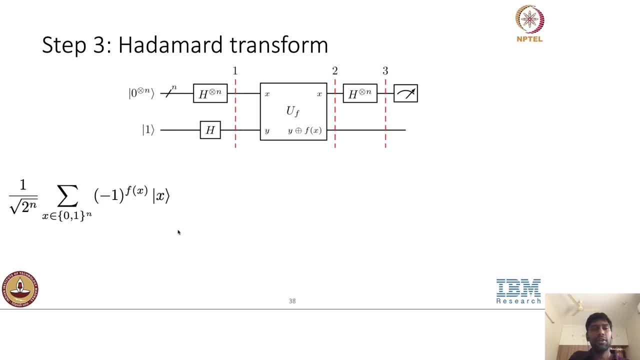 So now we have this state at the end of step 2.. We have 1 over 2 to the n summation over x, minus 1 to the f of x- x. Now we apply Hadamard, the previous expression for this. 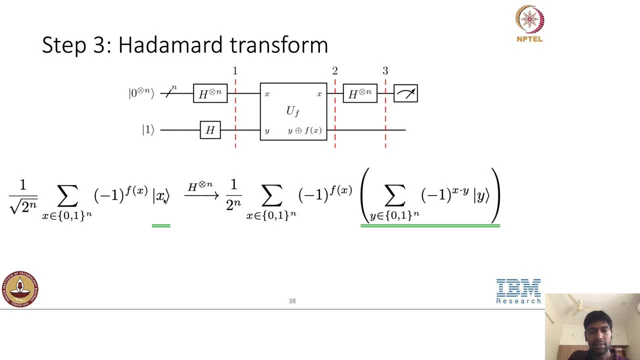 So each qubit x. so the x has the same thing as a. So earlier we said a, So this is x. it is just change of variables. this time here It is summation over all possible y minus 1 to the x. dot y get y. 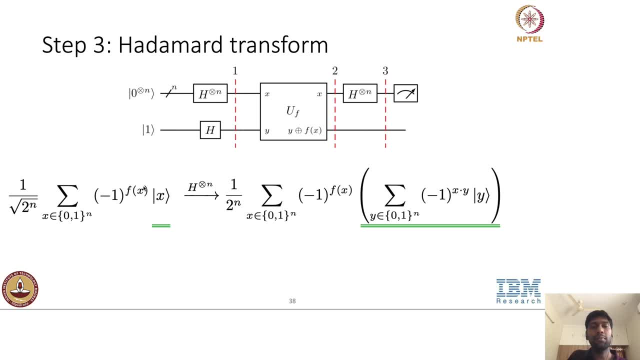 So we have Hadamard applied on this qubit general n, qubit variable x, and that gets transformed into summation over all y minus 1 to the x dot y 1. This expression now gets rewritten as follows: So we have the summation over all x and summation over all y flip and then 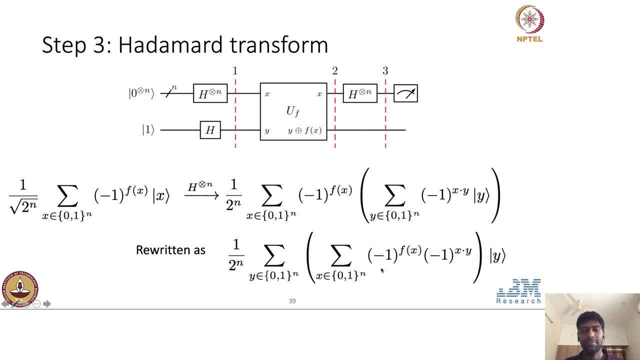 we just move this minus 1 to the f of x inside. We will expand this expression and then see how it gets the result that we want later. but I will just keep this rewritten expression here before we move to the next step. So the last step is just measure the first n qubits. So once you measure the first n, 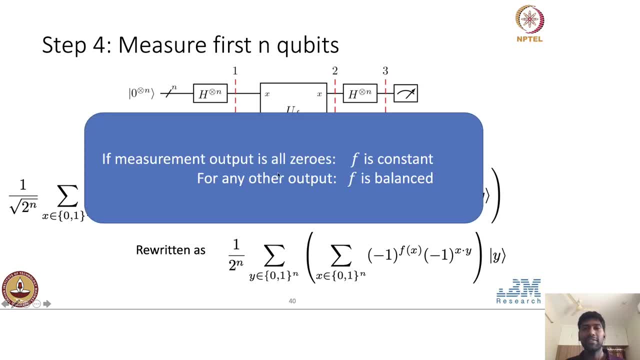 qubits. that is all about it. So if f is a constant function, then the measurement output will be all 0s. So at 0 to the n, all n qubits will be measured to 0.. If it is not all 0, that is output. if 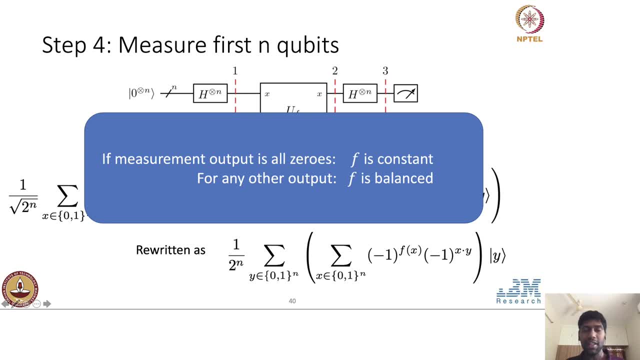 any of the bit is 1,, then we can conclude that f is a balanced function. So we can keep the same thing like this, Starting with engineer Mat Carolina. we will just derive this how we arrived at this, but that is all about it. These are 4 steps that we need to do. First is apply Hadamard on. 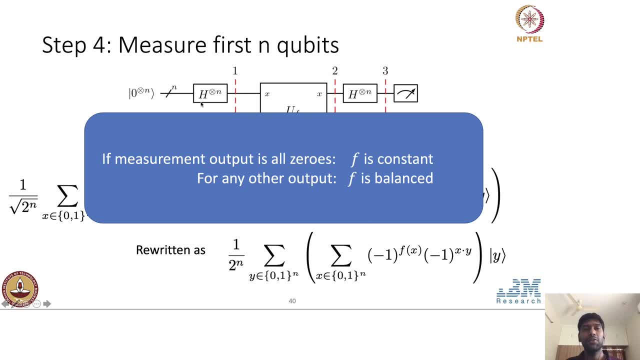 all the input qubits or even before that step 0, we prepared, and all 0 are the first n qubits to be 0 and the last qubit to be 1.. And then we apply Hadamard on all the qubits and then 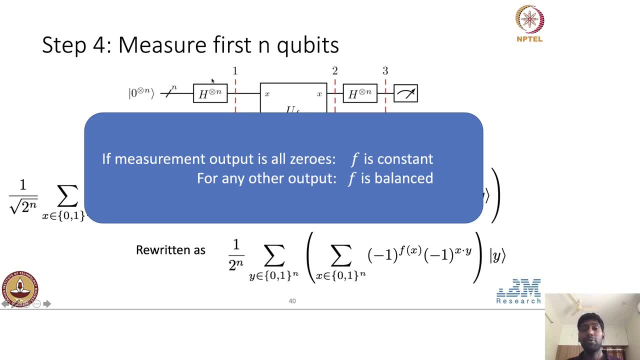 we apply the oracle. I mean they provide this what we prepared by applying Hadamard as input to the input oracle in order to darken the calculator code. sometimes, as we article, and we apply a Hadamard to the first in qubits again and we measure, that is all. 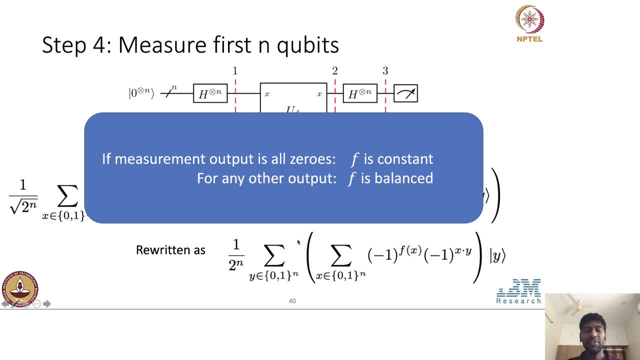 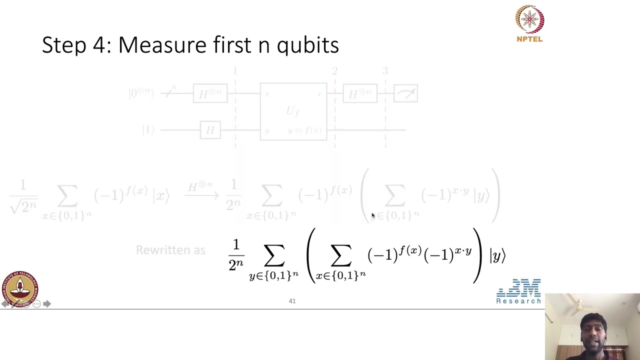 about it. I think the crux of it we have explained before, but I mean in term, like phase kickback and the Hadamard operation. one step that is remaining is how this expression, when we measure it, how this n qubits we measure it, it will give the output as we desire. 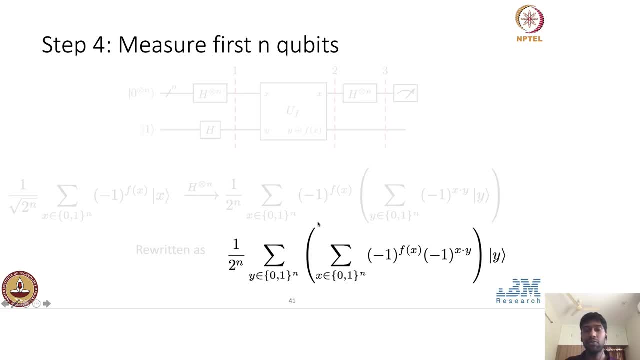 Let us focus on this expression In particular. we will focus on the one that is inside brackets. We will prove in the next slide that this expression, if we focus on the all 0 state, if you focus on the all 0 state, if you focus on the probability, this is the probability. 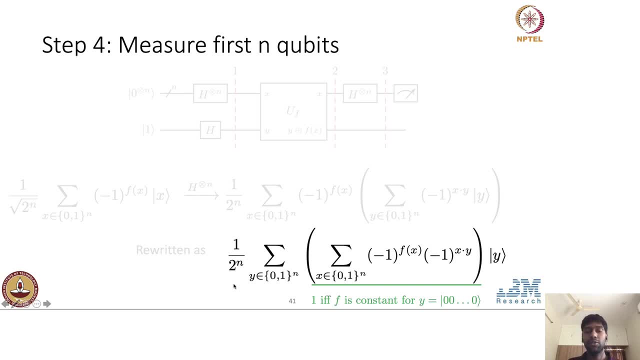 with respect to all 0 state, Because we have 1 over 2 to the n summation over all y this. So, if you focus on the probability for the all 0 state, we will see that if f is a constant function, the summation will. 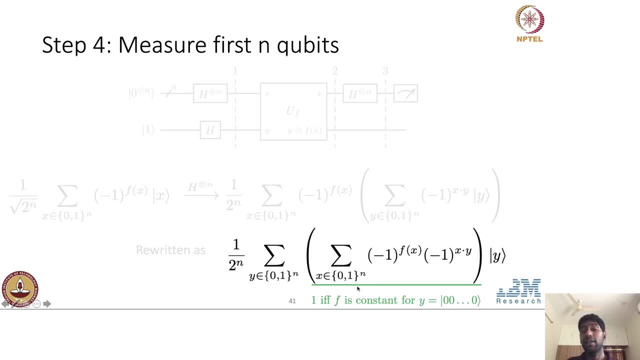 be evaluate to 1.. But if f is a balanced function, this summation will always evaluate to 1.. to 0 for the all 0 state. we will just see this. So this is the expression, same expression as this inside the brackets, and since we focus on the all 0 state, we substitute y equals. 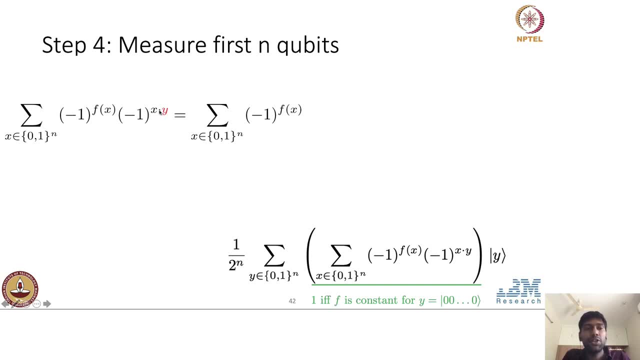 0.. So the dot product x, dot y is 0 and minus 1 to the 0 is 1.. So we have this expression summation over all x minus 1 to the power f of x. Just look at this carefully. if f of x, if f is a constant function, f of x is always. 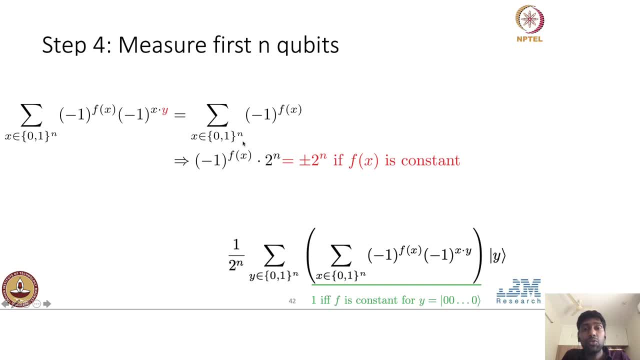 0, which means that its summation over all x minus 1 to the power 0,, which means it is plus 2 to the n. or if f of x is a constant 1, then it is minus 1 to the 1, which is minus. 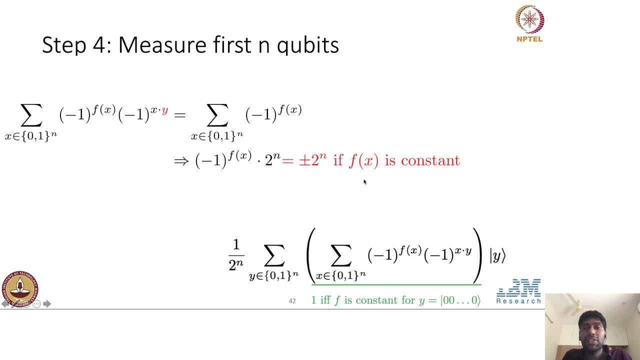 1.. So essentially, if f of x is a constant function, then we can just move minus 1 to the f of x. I mean, we can just write it as minus 1 to the f of x times 2 dot n. 2 to the. 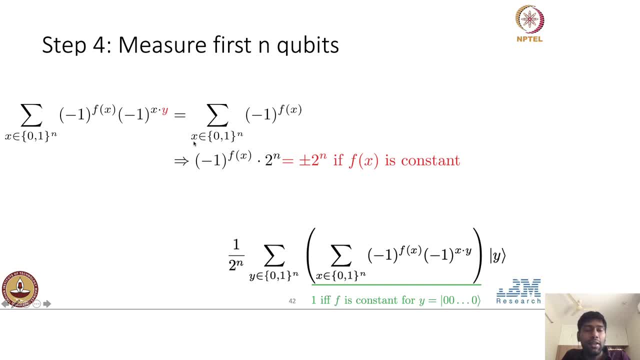 n because there are 2 to the n possible values for x and since f of x is a constant function, independent of what the x will be, it is just minus 1 to that constant value times 2 to the n. Essentially, if f of x is a constant 0, it is plus 2 to the n if f of x is a constant. 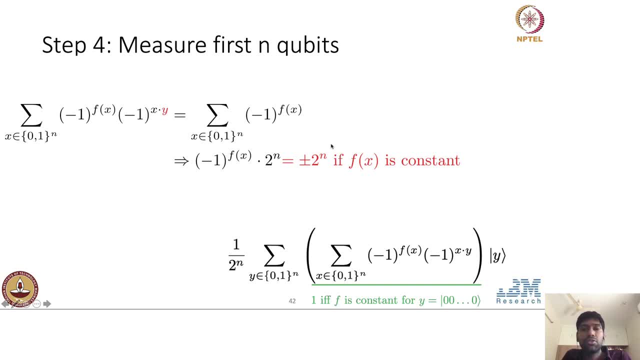 1,. it is minus 2 to the n, but essentially it is plus or minus 2 to the n. The modulus of it is always like 1, because we had this 1 over 2 to the n. So the modulus of this. 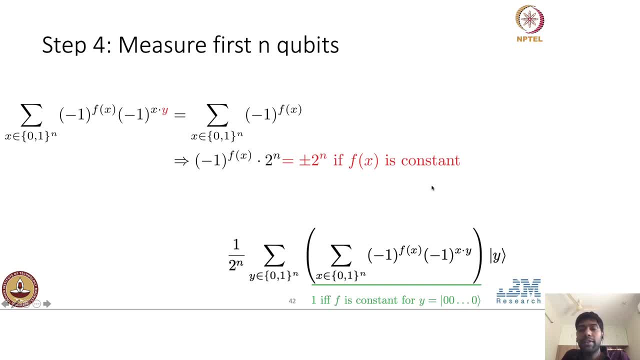 the probability for the all 0 state is 1,. if f of x is constant. What happens if f of x is balanced? If f of x is balanced for half of them, so for 2 to the n divided by 2 of them, we will. 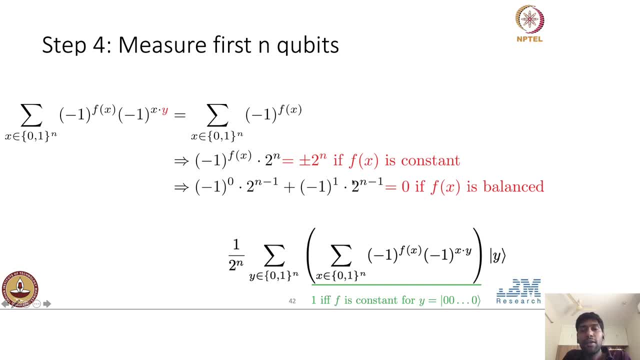 have minus 1 to the power, 0, because f of x is 0.. For the other half, f of x is 1, f of x is 1.. So we have minus 1 to the power, 1 times 2 to the n by 2.. Summation of this. 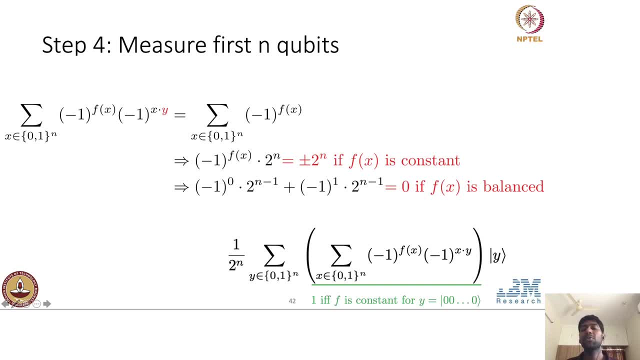 is 0. So for the all 0 state, if f of x is 0, then we have minus 1 to the power, 1 times 2 to the n. F of x is, if f is a balanced function, we get 0, and if f is a constant function. 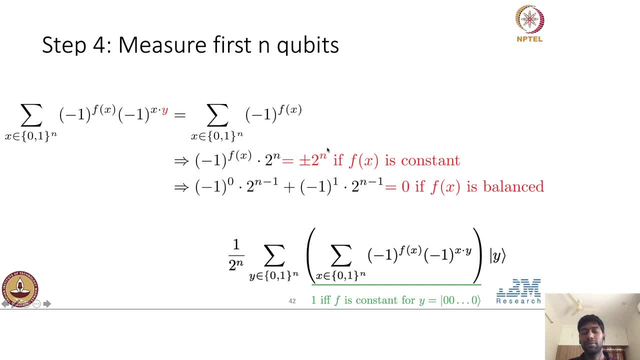 we get 2 to the n, divided by 2 to the n, is 1.. So that is what I summarized. as for the all 0 state, the probability of getting the all 0 state, which is this expression, is 1, if, and only if, f of x is 0.. So the probability of getting the all 0 state, which is this expression: 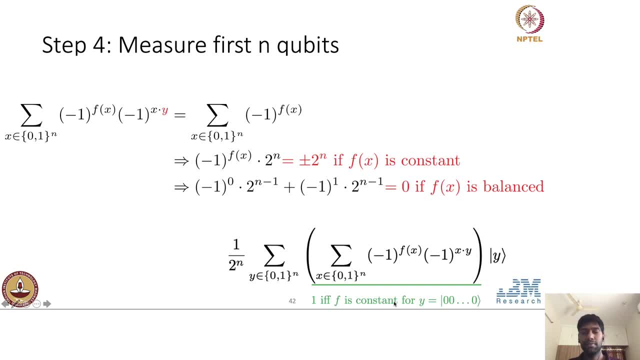 is 1.. So that is only if f is a constant function. In fact, it is more strong: it is 1 if f is a constant function and 0, it is not even something between 0 and 1, it is 0 if f is. 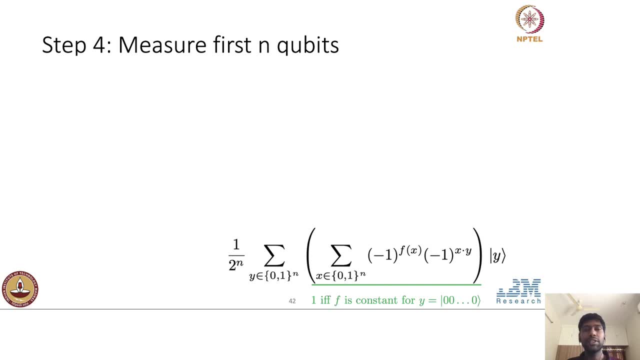 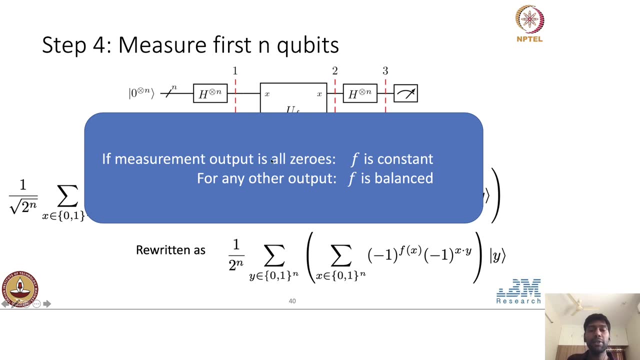 balanced. So this is what led to us to claim this previous expression. We said that if f is a constant function, the measurement output is all 0s, but if f is a balanced function, it will be anything but all 0s. We do not care about what that is, but if it is not, 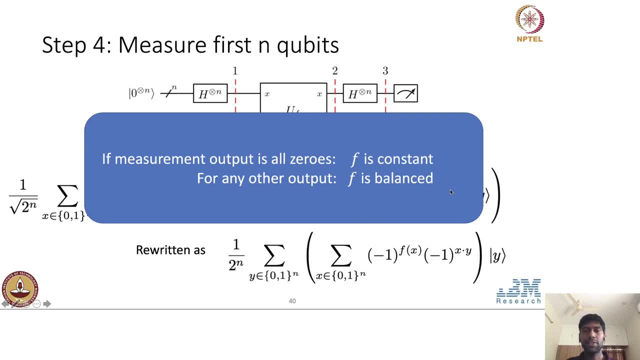 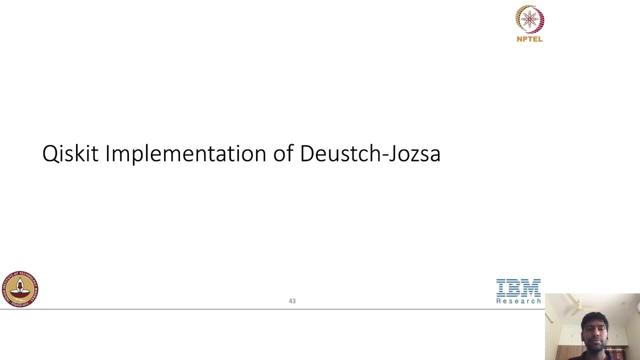 all 0s. we know that f is a balanced function. there is no gap in between. So that is the explanation of the Deutz-Jozsa algorithm. Now we will get to see the Qiskit implementation of this Deutz-Jozsa algorithm. We will go to the Qiskit. 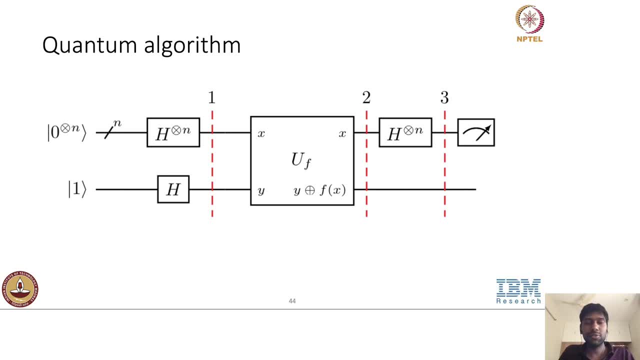 Qiskit, The page Qiskit Composer to go to the implementation. And remember, these are the four steps that we have. The first step, I mean even step 0, 0th step, will have inputs, that is, will have n qubit, input 0, and then n plus 1th qubit to be 1, and then we will apply Hadamard right. 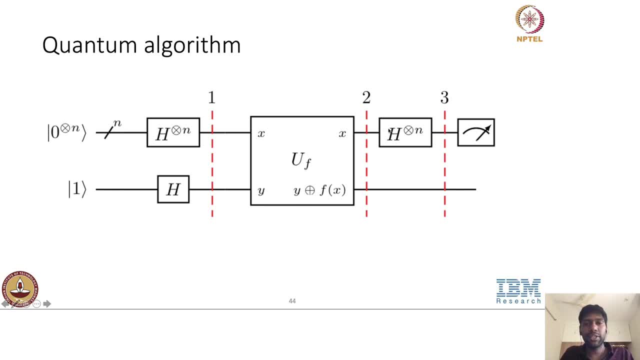 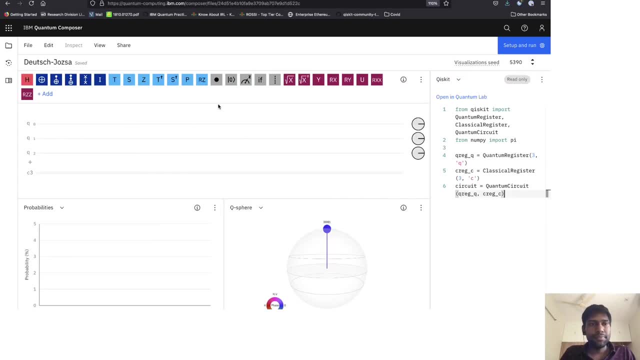 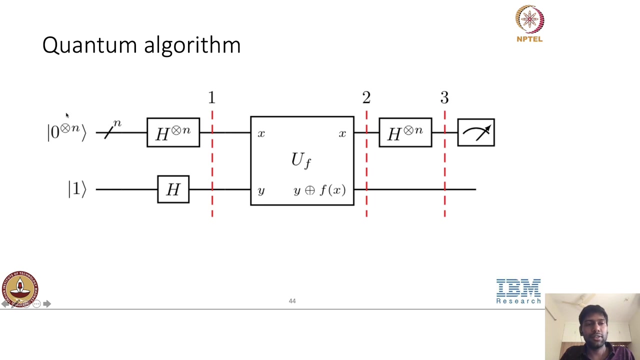 And then we apply the oracle, We apply Hadamard again on the first n qubits, And then we measure. Let us look at it step by step. First, let us say we will choose n to be 3. So we will have Q0,, Q1 and Q2 as the first register, like this corresponding: 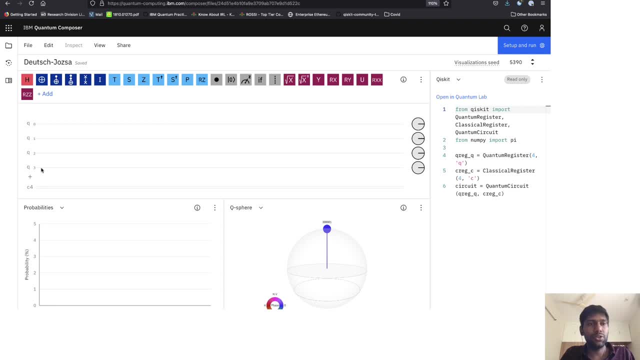 to 0 and then the last one to be 1, it is Q1.. assigns has the initial state to be 0. So q 0,, q 1, q 2 are by default 0. So I will. 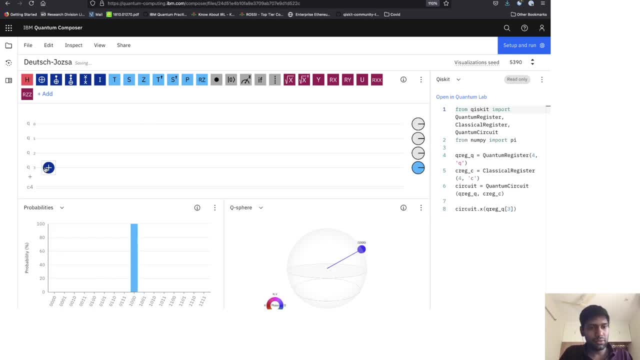 just make the last qubit as 1.. If you just look at it, I mean, this says that it is all 0 0, 0, followed by 1.. So you have to read from here to here, right to left. I will just. 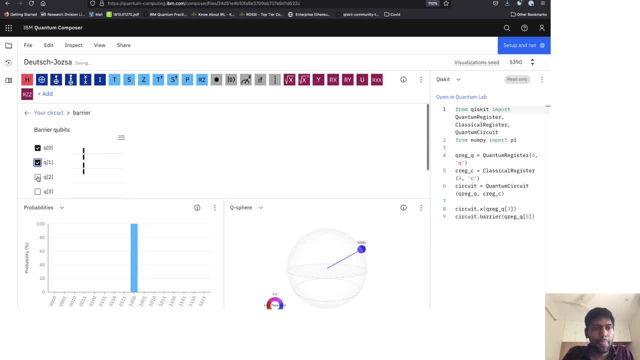 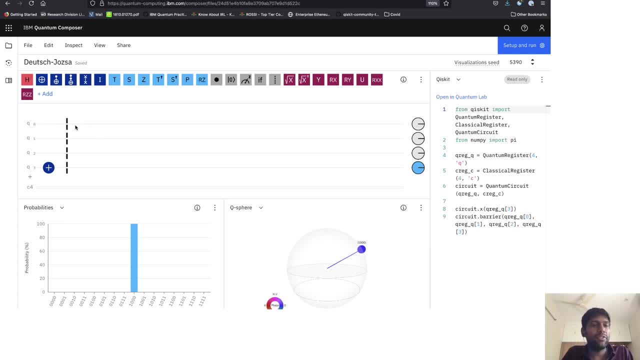 it has nothing to do with enforcement. pelos. We have 0 0 0 1.. Some players have 0 0 0 0 0. So it has nothing to do with the computation right after the barrier. It has nothing to do with the ensemble: 4.. But seg. up, So never, Let us let you Now. this is our third term, So here is the second term- to find the error code. This here it says: the error code is 0 1, 1.. So here we have. 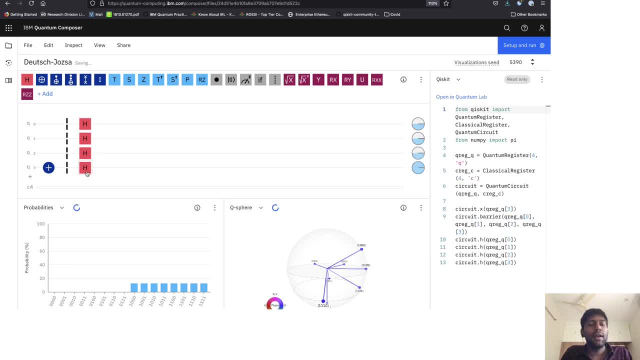 Q 1,, Q 2 and Q 3.. Let me add a barrier again. So now we can easily see that if, given that we have applied Hadamard and all of them, it is equal superposition of all qubits, Since 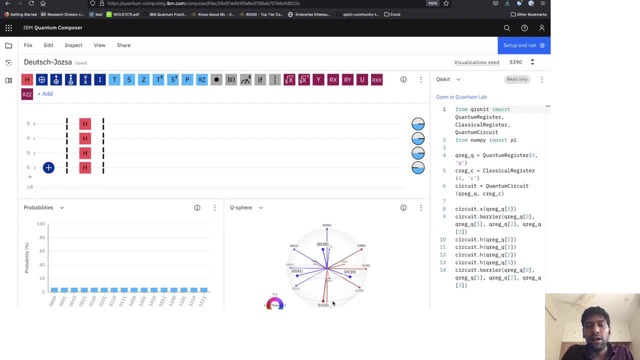 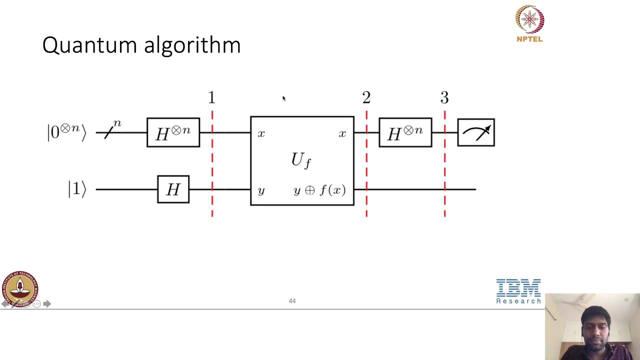 there is a minus here. there is. some of them have phase associated with them, but for now I think let us just go. So the next step is the implementation of an article. When I first motivated article, I told you guys that it is an abstract notion. 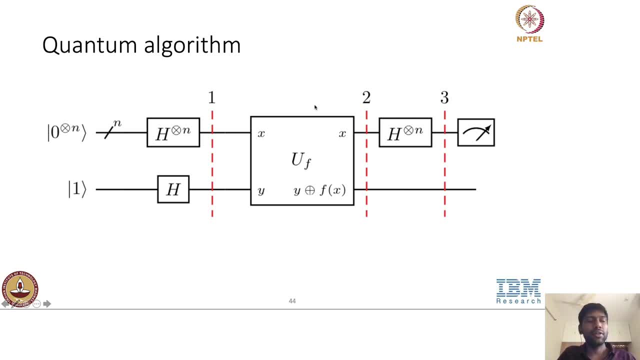 we are using it to separate- I mean differentiate- the complexity of two algorithms or two complexities, Two classes of functions, so on. But now I mean here we are looking at the instantiation or implementation of this quantum algorithm. So for this purpose we will look at how to. 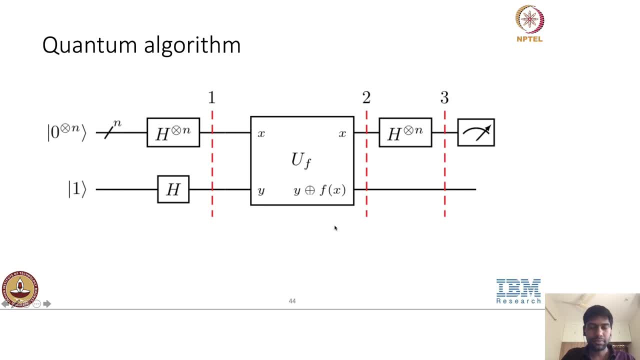 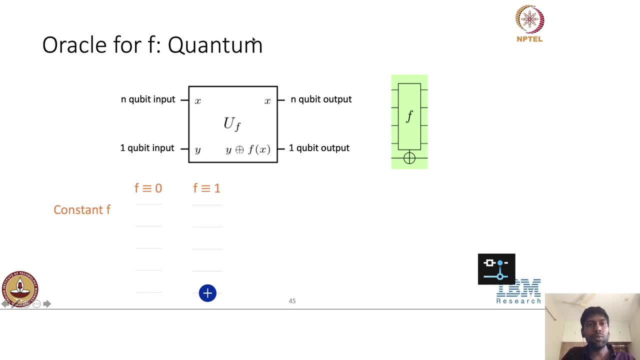 implement or instantiate this article. So just to recap, the quantum article for f is as follows: it takes an n-qubit input x and 1-qubit input y And then now has a n qubit output x and 1 qubit output y plus y, xor f of x. So, as I described before, 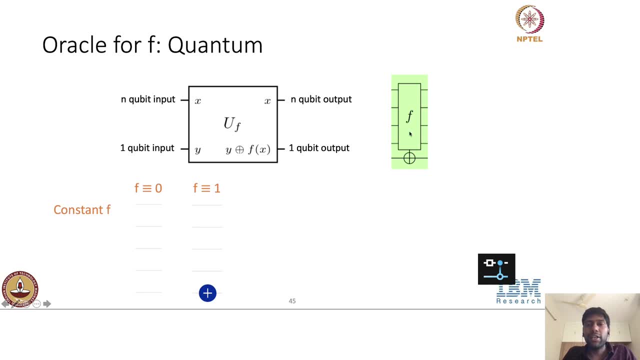 it is equivalent to a conditional, not where the condition is f of x. So now, how can we instantiate this article? Actually, it is easy, if it is a constant function. So what does it mean that f is a constant function, f of x is constant irrespective of what x. 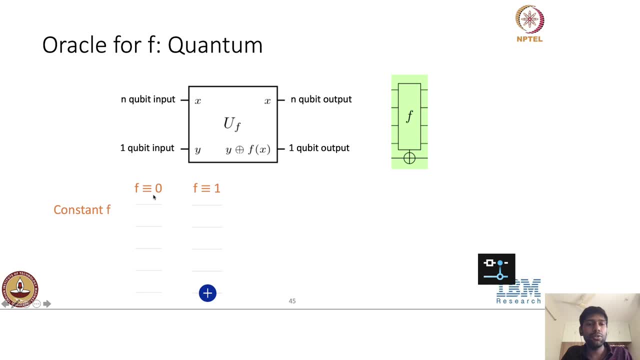 is. So the constant can be 0 or 1.. So what does it mean if f is a constant and the output is 0?? That just means that f of x is 0 always, which means that on input x, y we already get, we also get the output to be x and y. 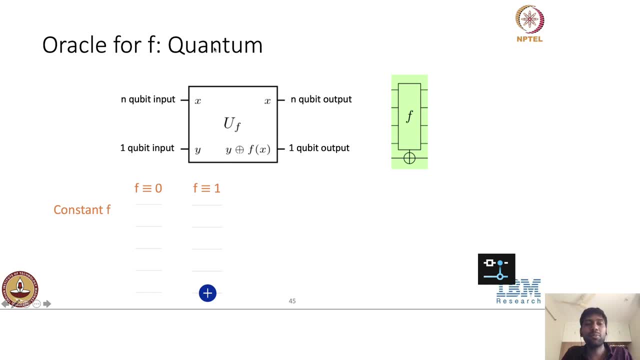 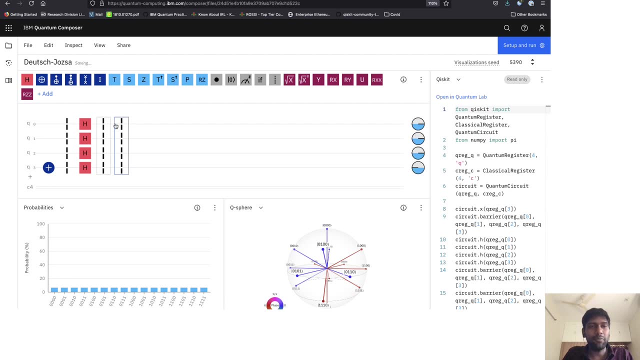 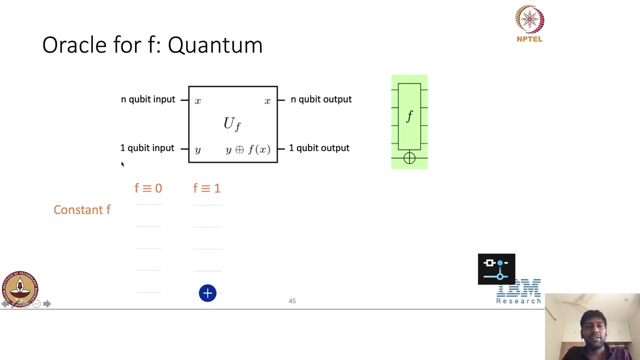 which means there are no gates. do you upgrade applied to implement this? So, essentially, if I say that in step 1, if I say that there is nothing, no gate that is applied, I mean no gate that is applied here. that is equivalent to applying a constant article. 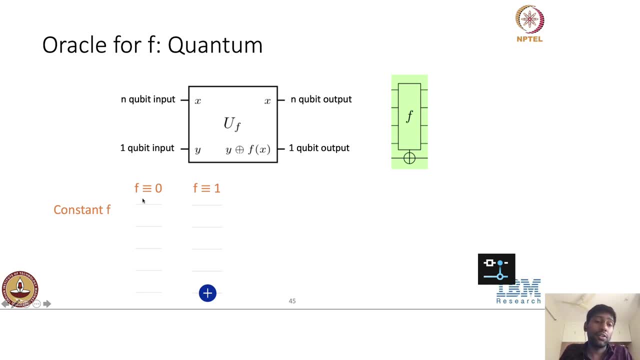 where the constant is 0,. constant article for a constant function f where the input is 0, where the output is 0.. On the other hand, if it is a article for a constant function f where the output is always 1, what does that mean? on input x and y. 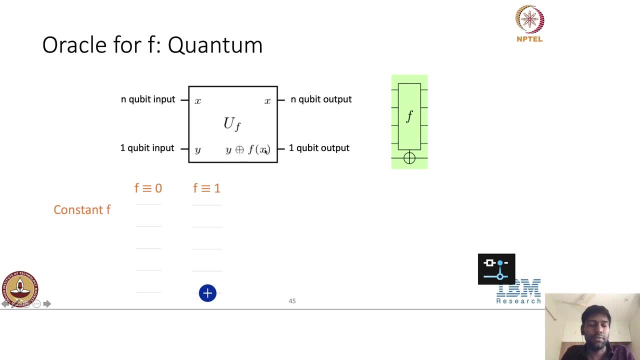 we get output as x and y. x of 1, this is y being flipped, So we just apply the x gate here. So this is the notation for x gate that Qiskit has. So we just apply the x gate in the last position. 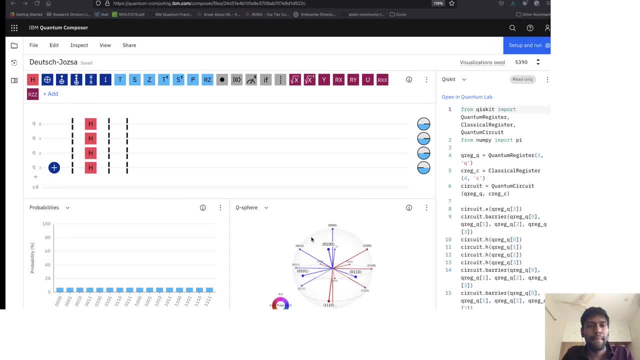 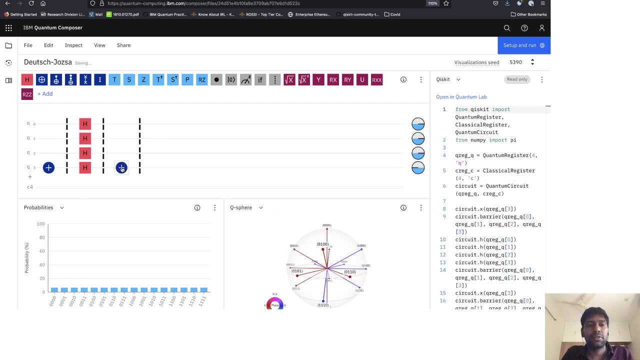 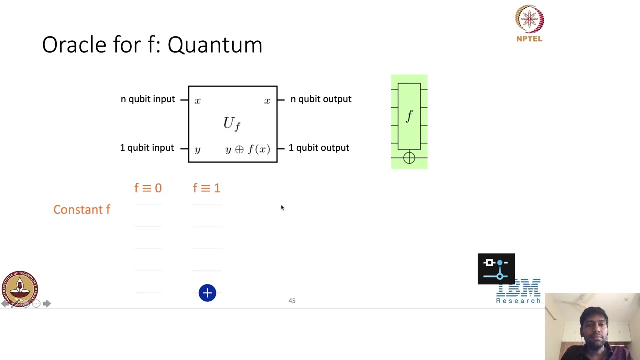 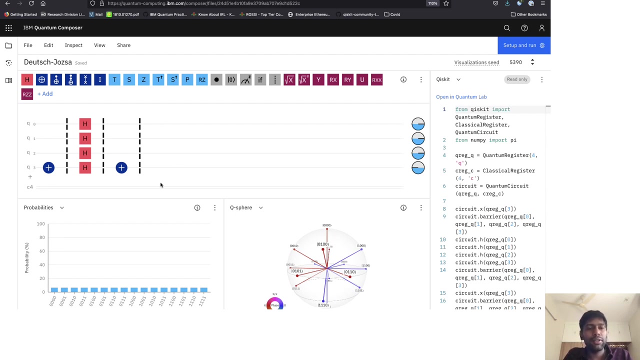 there is nothing else to be done on the other gates. So if I were to implement constant article for a function which always outputs 1, then it is. this is the article corresponding. Let us go to the balance thing. later We will see what happens when we apply constant article. So the promise from the expressions 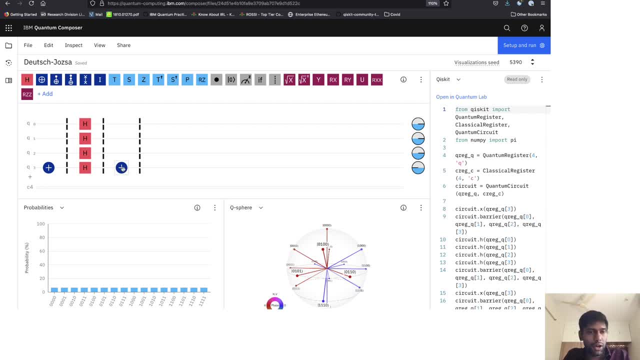 that we derived. what I told you is if we apply a constant article, then the all 0 state. I mean we have to ignore the last qubit. that can either be 0 or 1. But the first 3 qubits. once we apply the Hadamardian measure. it should always be in that. 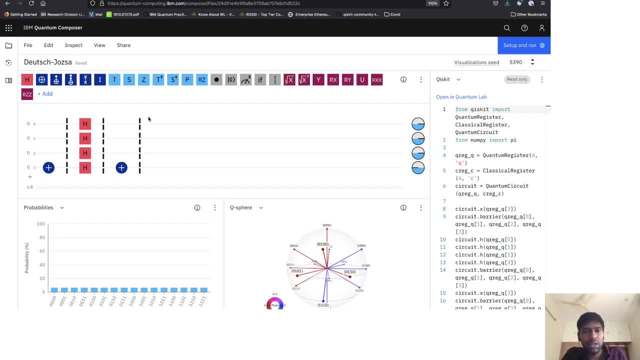 So the first 3 qubits should always be 0 if it is a constant article. Let us look at how it works. So this is step 1, step 2, and let us look at step 3.. Step 3 is applying the Hadamard on the first 10 qubits. So on the first 3 qubits, 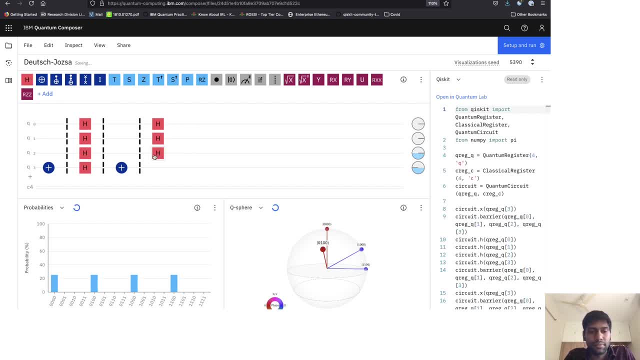 I will apply a Hadamard, Let me apply a barrier again, just to demark it. So let me apply a barrier again, just to demark it. All, right now, let me measure the first 3.. Oh, sorry, So this is the first measurement, measuring the second. 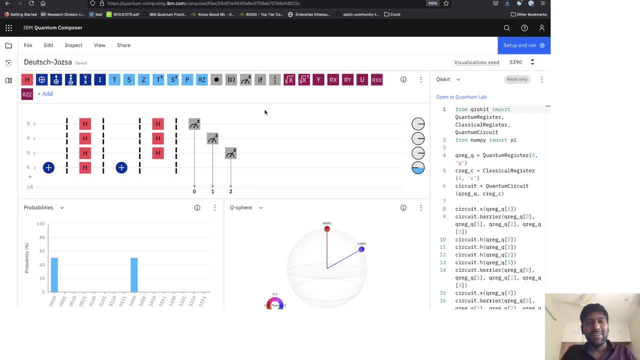 and measuring the third, Cool. So what do we get? The final state that we get is 0.. For the first 3 qubits, the measurement is always 0. I mean, it boils down to that state. It still is split between 2 because we did not. we have not measured the last one. 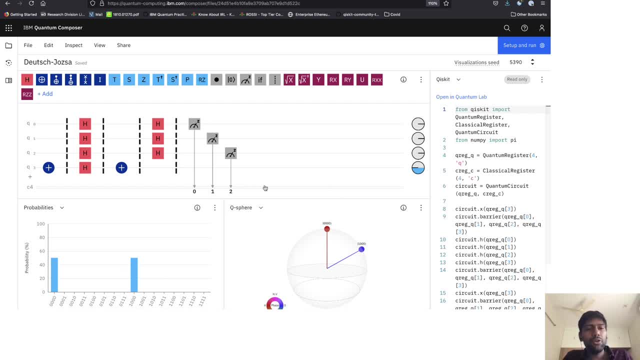 So that can be. we do not really care about it as a part of the Deutz-Joseph algorithm. But here it says that it is either 0 or 1, with probability half. But we do not really care about that. We care only about what is the output for the first 3 qubits. 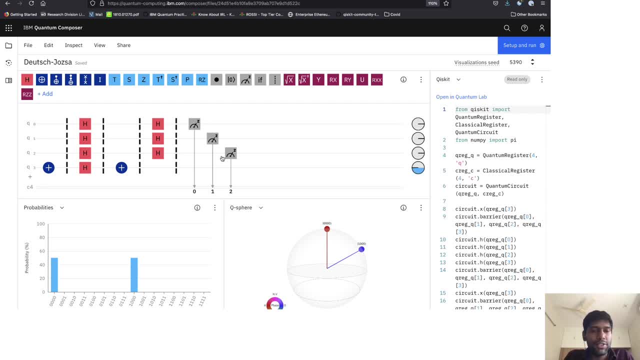 That is 0, 0, 0, 0, 0, 0. So it is always 0, 0, 0.. Let me delete this. So if I delete this execute, it essentially means an article for a constant function, for f equals 0. 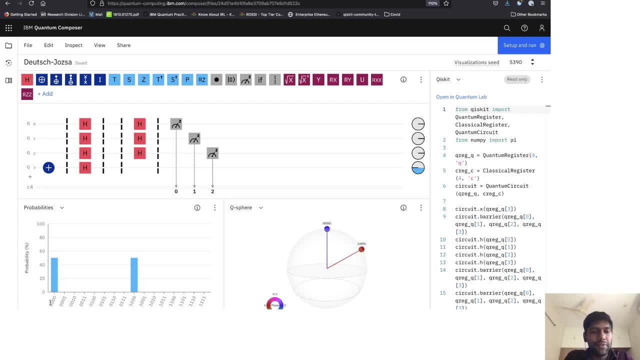 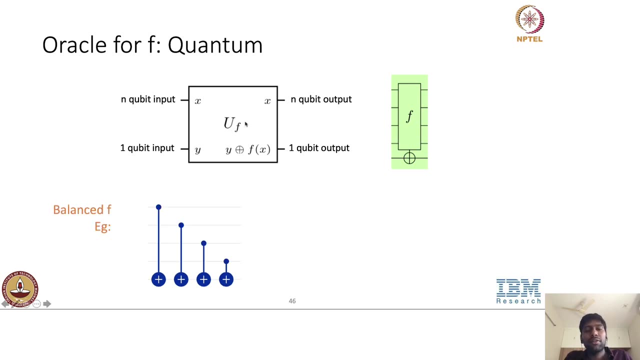 Again, we get the same state, which means that the first 3, bits after measurement are always 0. So this is what we expected if it is a constant article, article for a constant. Now let us look at how to implement a balanced function. So what does? 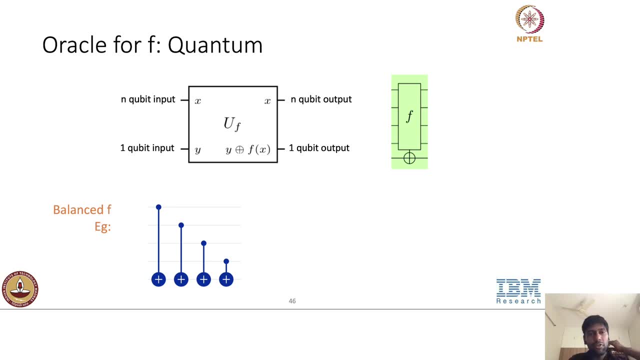 a balanced function mean. So there are multiple instantiations for it, for implementing an article for a balanced function, But this is one simple way of looking at it. So one example for a balanced function. So this is a simple way of looking at it. So one example for a balanced function. 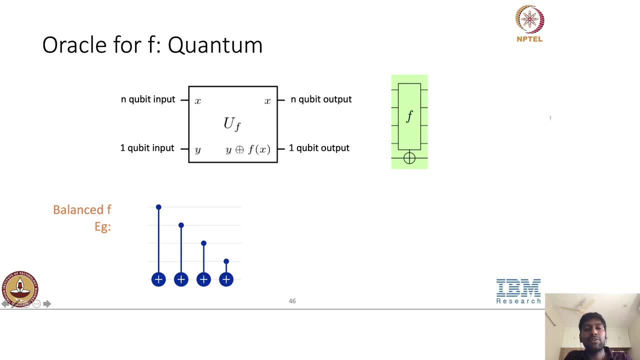 is that its x r of all the individual qubits. So f of x is x, 1 x, r, x, 2 x, r x 3.. There are 3 qubits: x, 1 x, r, x, 2 x, 3.. 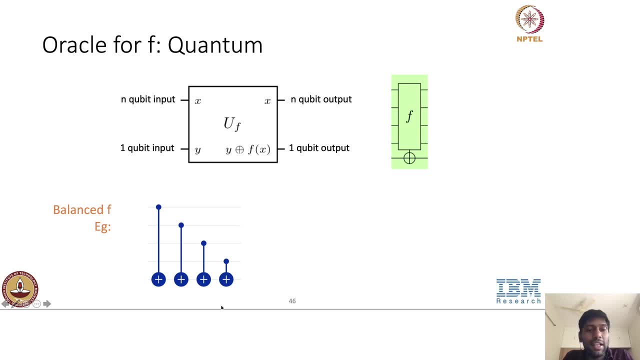 So it is an exercise for you guys to check. why is this a balanced function? but for any qubits, If you work it out, you can see that many n 0, 0, 0, 0.. If I make an article for a balanced function, 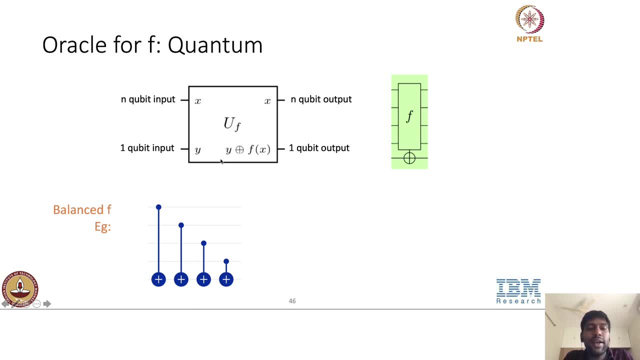 that is a balanced function. But for any qubits, if you work it out, you can see that the first, that for any number of qubits this is one example of a balanced function. You can also have many other instantiations of a balanced function. I mean, after all, there are like 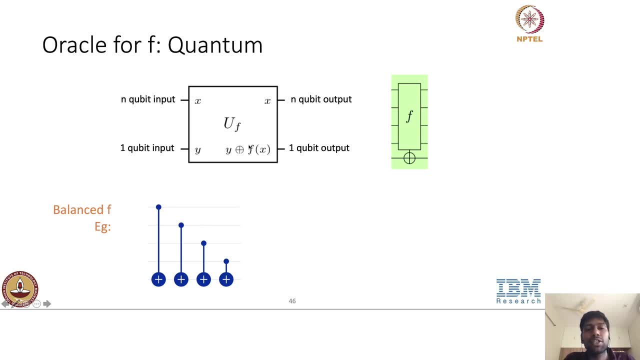 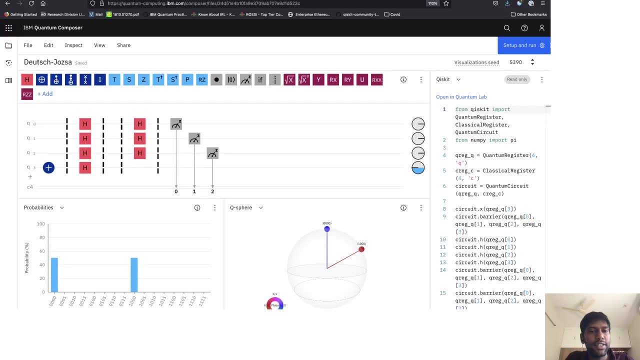 many possibilities for making this function output 0 for half of the inputs and 1 for half of the inputs. This is just one degree of doing it. So let us see if I- for now, you guys just trust me that this is an oracle for a balanced function. and let us see how. 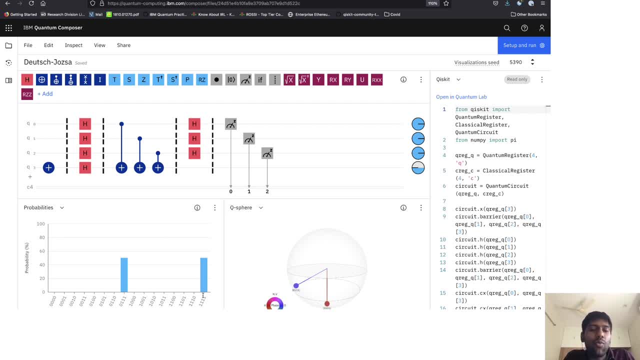 that. what do we get? We get a state here. actually, we are getting 1, 1, 1, but it can be anything. The only thing that matters for us is that there is 0 probability for 0 0- 0 token either. 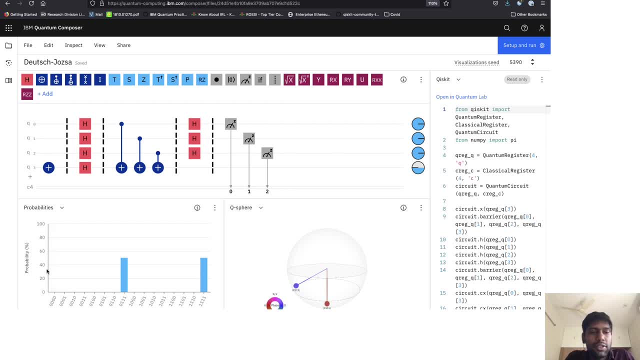 it is this. So there is 0 probability for this state or this state. It is about the same. even if we have the x gate, that is applied To any of the qubits. So any of these qubits, it is still an oracle to a balanced function.